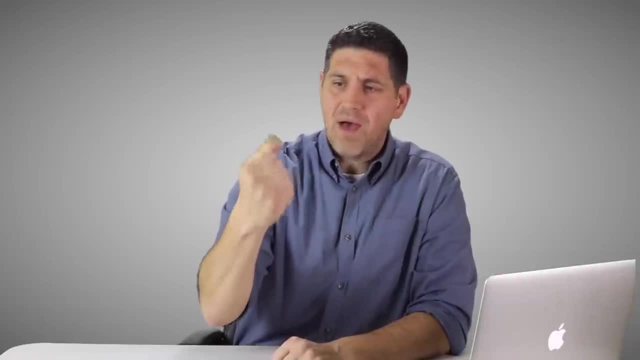 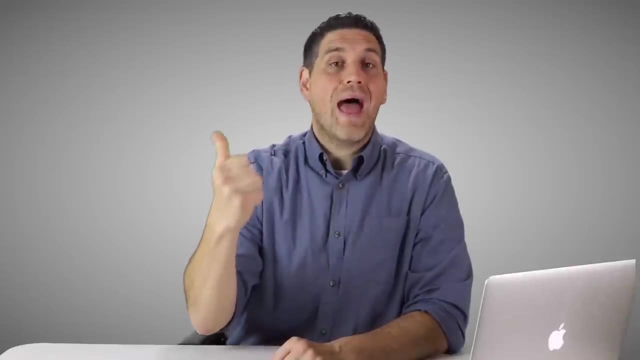 Take out your fist and do this: Thumb out, and then pinky out, Thumb out and then pinky out, Just like this. Do this a couple times. Okay, Perfect, All right, That was round one. Okay, Round two. 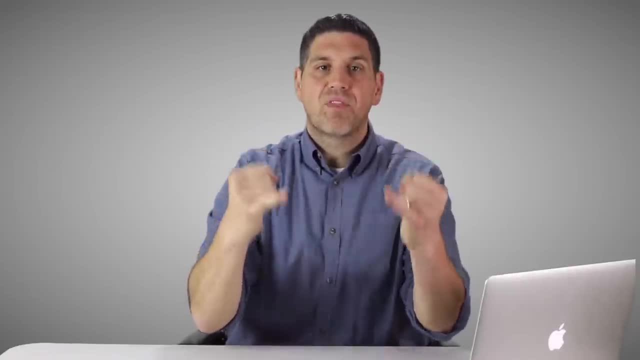 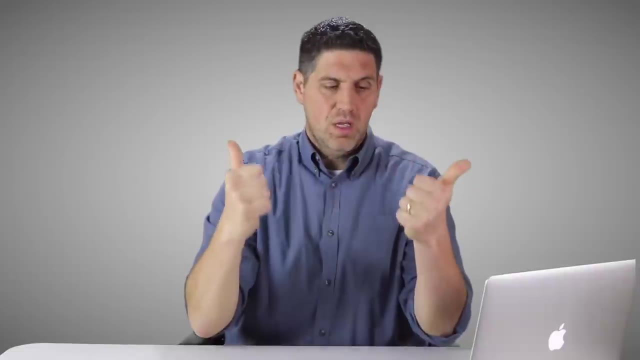 I want you to do the same thing, except with both hands. So, pinkies out, thumbs out, Pinkies out, thumbs out, Pinkies out, thumbs out. Okay, Do this. All right, That's round two. All right, Here we go. Last one, Round three. I want you to pinky out, thumb out at the same time. 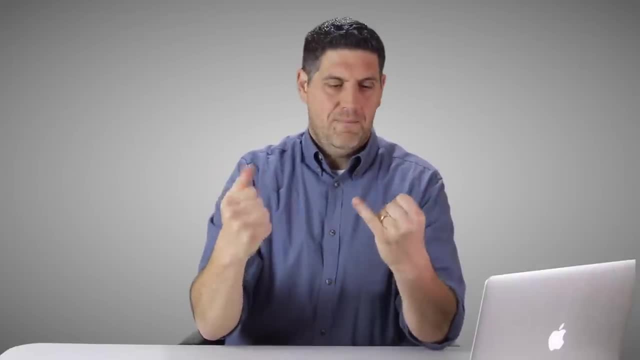 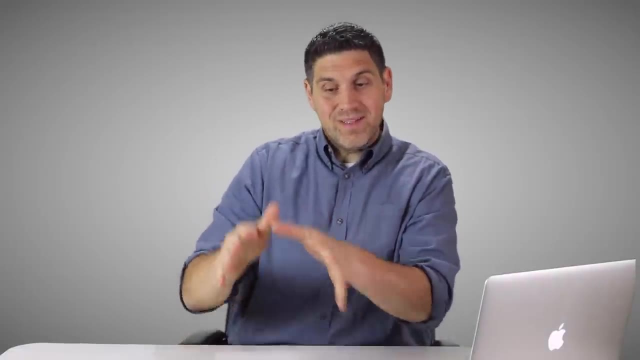 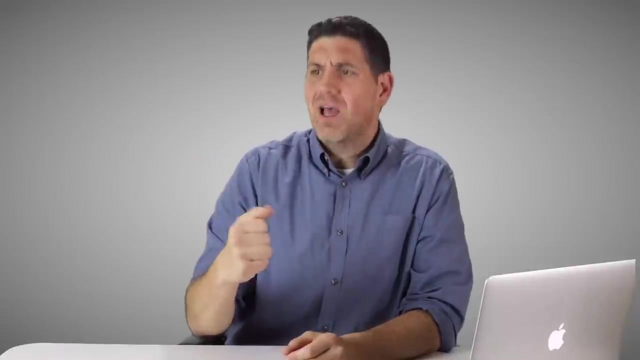 and then pinky out, thumb out, Just like this. Okay, All right, Try this Perfect. There's two reasons I'm making you do this. The first one is that economics is exactly the same way. It starts off really easy. There's going to be all these concepts You're like: oh, I totally get this. 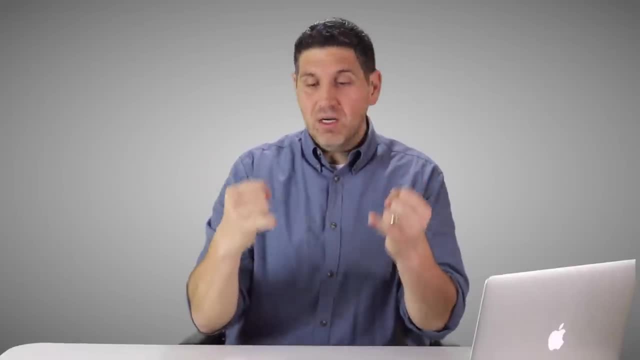 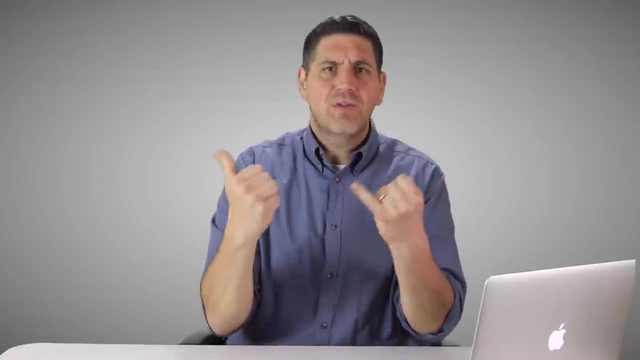 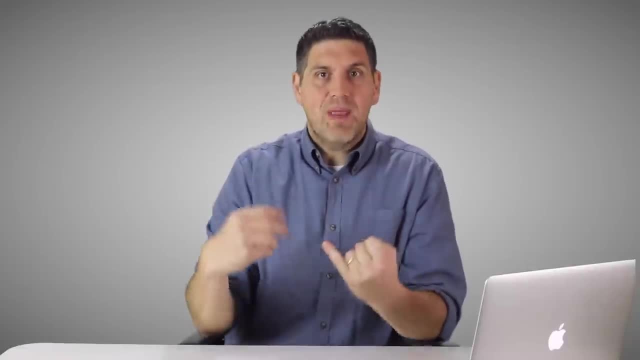 this all day long, but that doesn't mean that you're good at it. So if you're watching me and think, oh, he did that, I get it, It makes sense. Nah, nah, You got to practice And that's the. 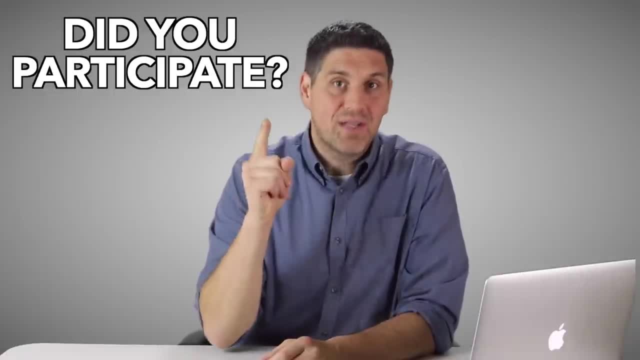 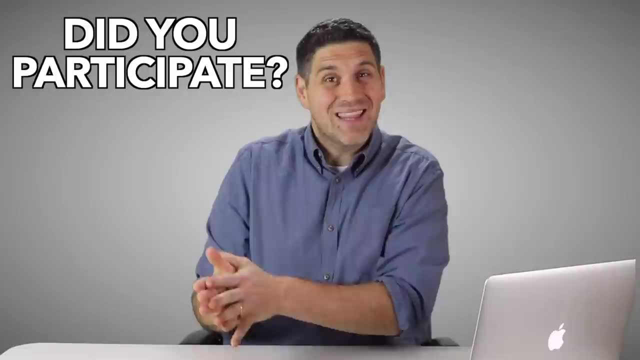 second reason why we're doing this: I want to find out if you can participate. So if you just watch me doing this and you didn't do anything at all and you didn't practice, you're probably not going to get the most out of these videos. You're not using them right. So when I say, okay, stop. 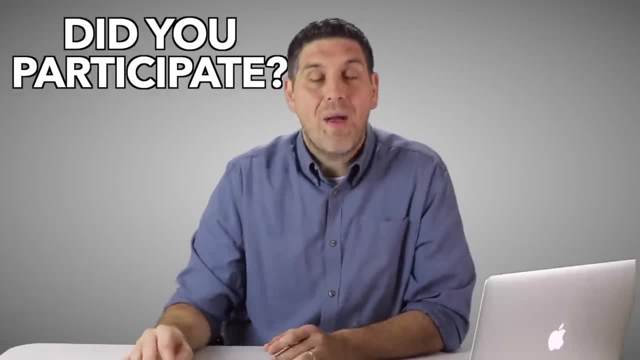 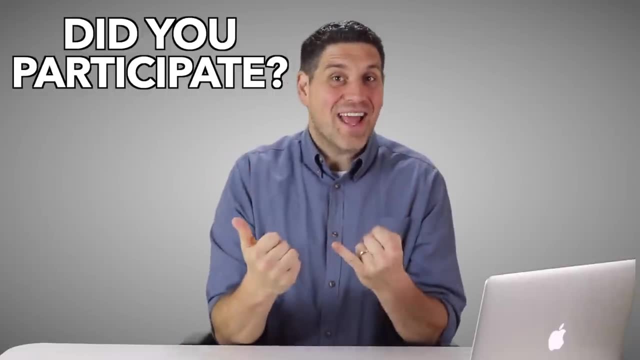 practice drawing this graph or try doing this in the ultimate review packet. stop the video and practice, because that means you're actually trying verifying, you're actually getting it. Remember, I'm really good at economics. I can explain all the concepts. I can draw those. 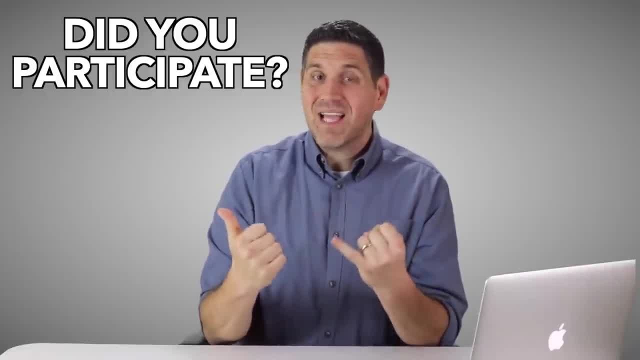 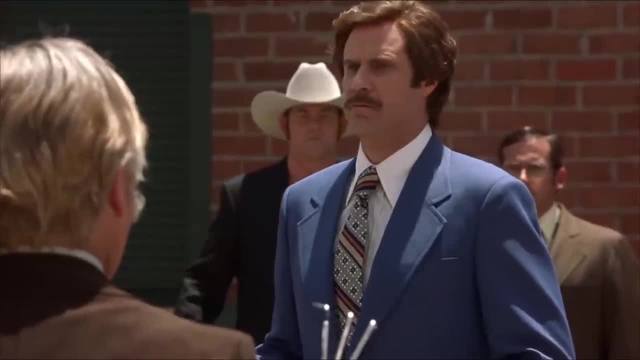 graphs and do those calculations really quick and it makes it look easy, but it's not going to be the same for you. You are going to have to practice. The point is: please participate, And that's it. Now, let's do this. We're going to start off talking about what economics is. It's? 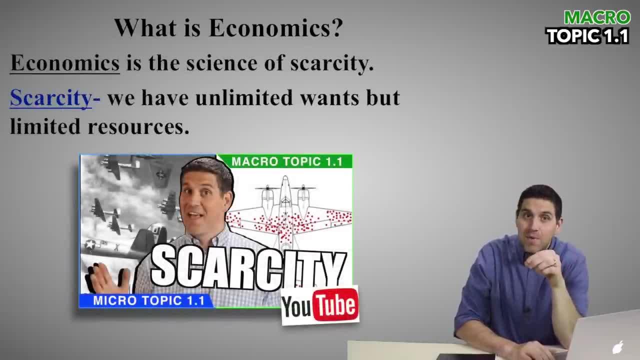 the science of scarcity. Scarcity is the idea that we have unlimited wants and limited resources. So in your class it's the first thing your teacher is going to talk about. Most people think economics is about money. It's not. It's about limited resources. So economics is how we deal with the 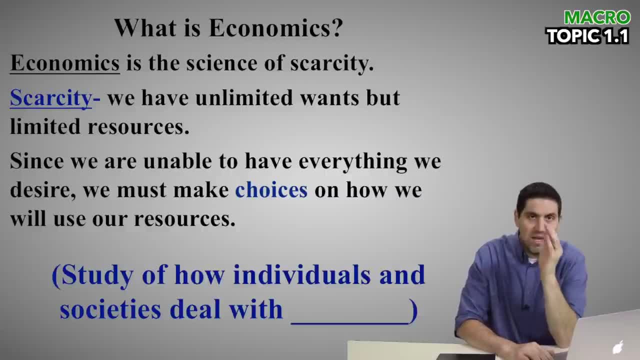 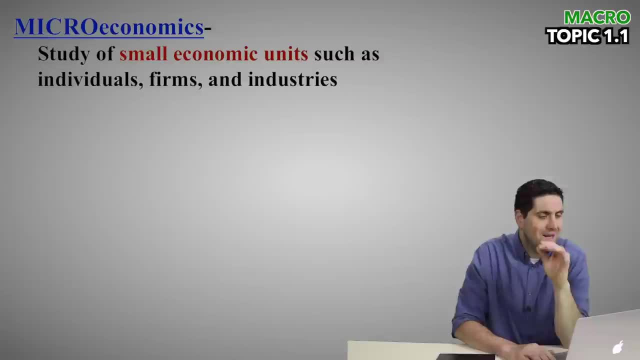 idea that we can't have everything and we're forced to make choices. It's really how individuals and societies deal with the idea of scarcity. Now there's some key terms I want you to go over. There's a difference between microeconomics and macroeconomics, and there's actually two. 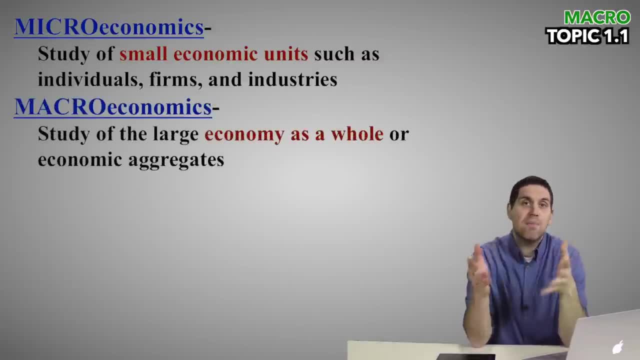 different courses. So if you're in college, you're probably taking micro or macro, and they're the same thing for the AP test. Microeconomics is the study of small economic units. So, looking at firms, you're probably taking micro or macro, and they're the same thing for the AP test. 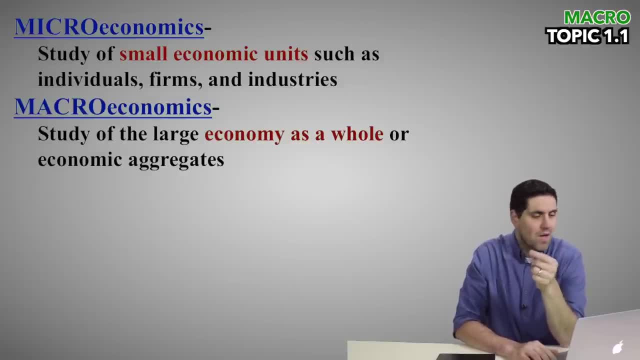 And they're the same thing for firms and individuals and their decision making and governments as well. But macroeconomics is looking at the big picture, the entire economy, like inflation and unemployment and gross domestic products and how the economy is doing Is there. 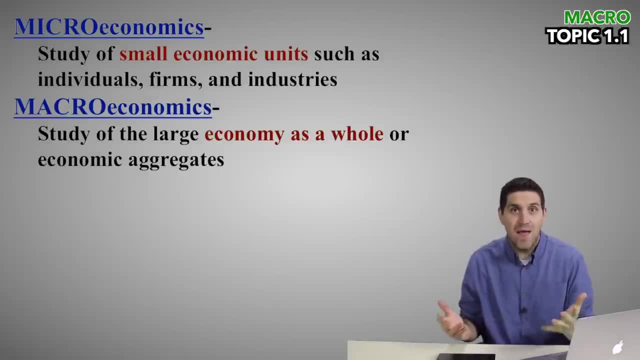 a recession. How can the government help to get out of a recession? Should the government help to get out of a recession? These are all concepts you'll see in macroeconomics. Trade-offs is another key concept. It's all the things you give up when you make a decision, but they're all the. 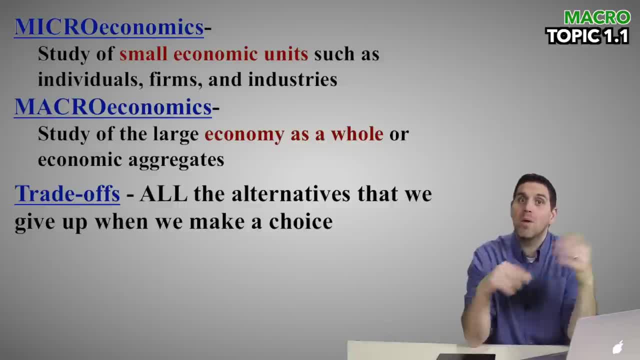 things, not just one. So what's the trade-off of watching this video? Well, you could be watching some other video. You could be watching some other video. You could be watching some other video. You could be hanging out with your friends. You could be sleeping The time watching this. 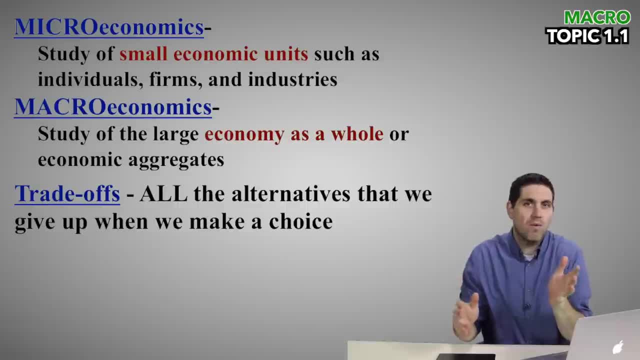 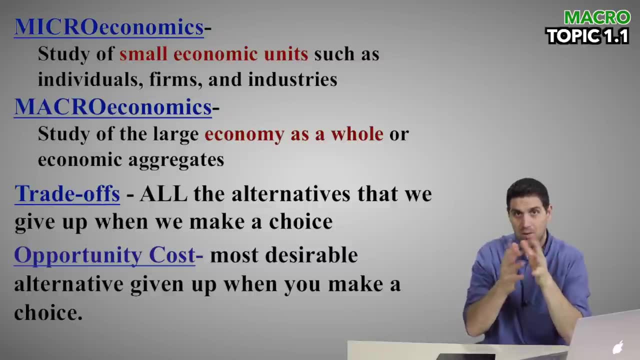 video has a cost. the things that you're giving up, but you can't do them all right. You can only actually have done one. The one best thing, the thing you gave up is called your opportunity cost. It's the most desirable alternative. when a choice is made Now, most people think: when we 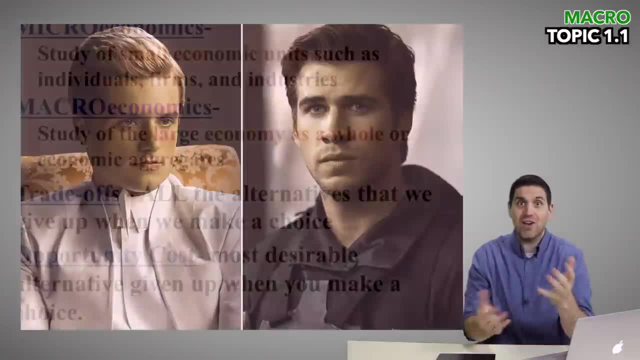 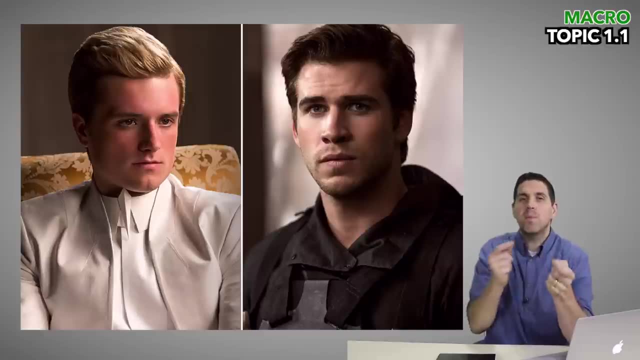 talk about costs, we're talking about dollars and cents. but it's not just that right. There's other concepts, For example, who you should date. You have to decide what's my opportunity cost If I date that girl, if I date that guy, who's the person I'm giving up by dating them? Now, 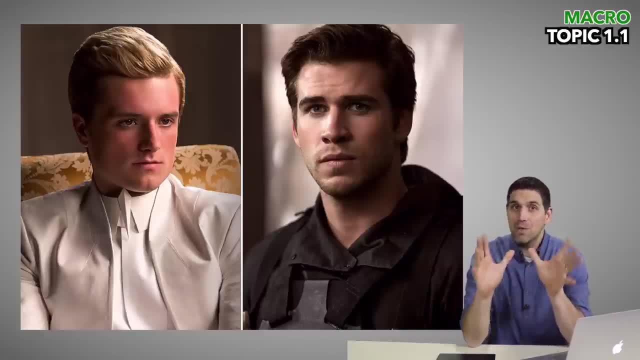 this concept is the most important concept in economics and, most importantly, it sets you up for what the point of the class is. This class will change the way you make decisions. It's going to enlighten your mind, to allow you to make better choices. Opportunity- cost is the key to 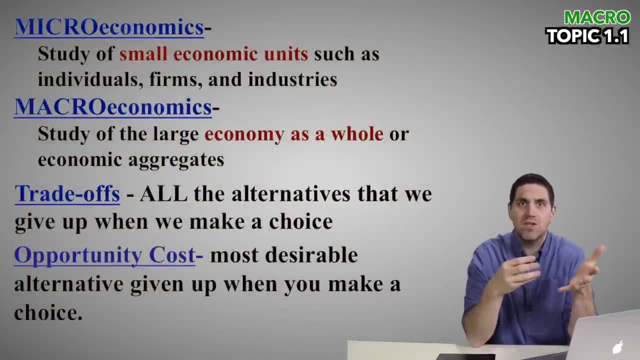 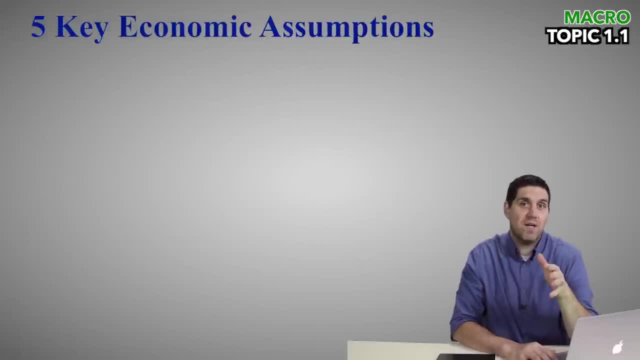 that Whenever you make a choice, you got to think of: well, what am I giving up to make this choice? So this happens for individuals, businesses, for the government, This idea of opportunity cost is huge. Okay, there's five key economic assumptions. I'm going to go over each one of them pretty. 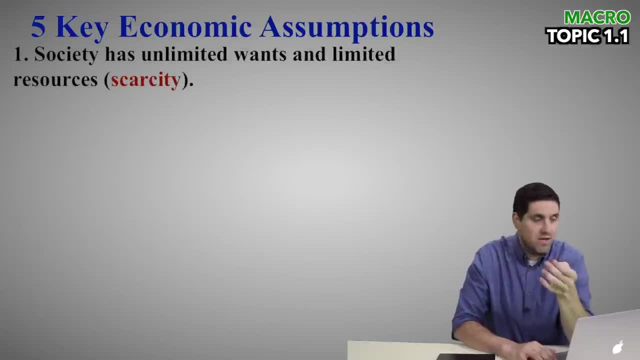 quick. The first one: all resources. All resources are scarce. We have unlimited wants and limited resources, and because of that we're forced to make choices. and everything has a cost. Your teacher probably already told you there's no such thing as a free lunch, right? So everything has a cost, something that you gave up. 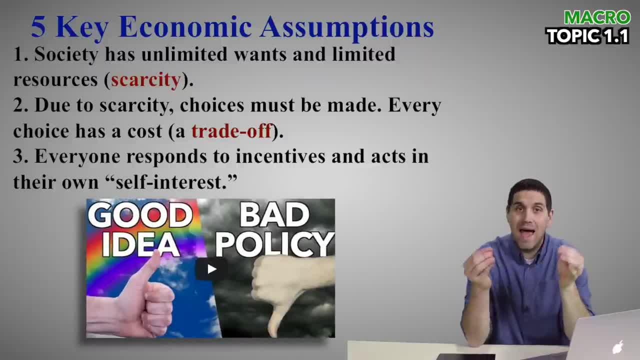 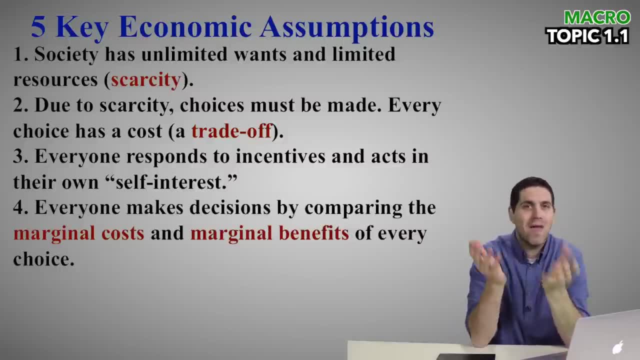 to get it. Everyone responds to incentives and acts in their own self-interest right. And then, for number four, everyone makes decisions by looking at the additional benefit and the additional cost of your decision. So you weigh the benefits and cost of every decision, And last one life. 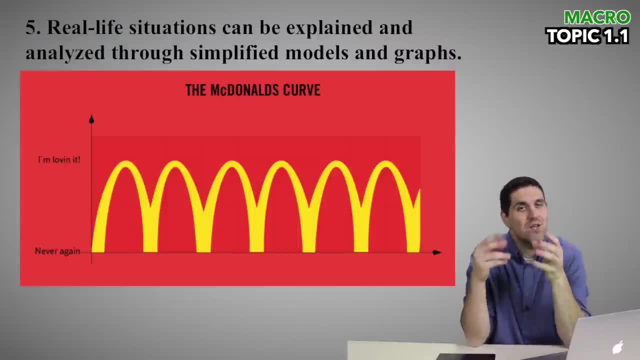 can be explained kind of can kind of with graphs. You're asked to explain life, You can explain the economy with graphs. It's not perfect, but you're going to see a lot of graphs in this class, starting here in unit one. There's a couple other key terms. 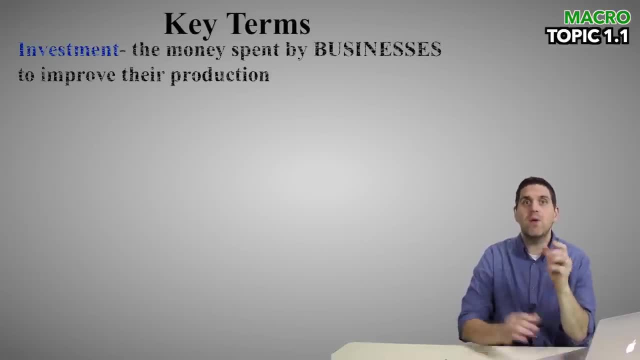 I want to cover really quickly. First one is the idea of investment. Now, when you hear the word investment, you think of stocks and bonds and retirement accounts, not in economics. In economics, investment is always when a business buys machines, tools and capital for their own business. So 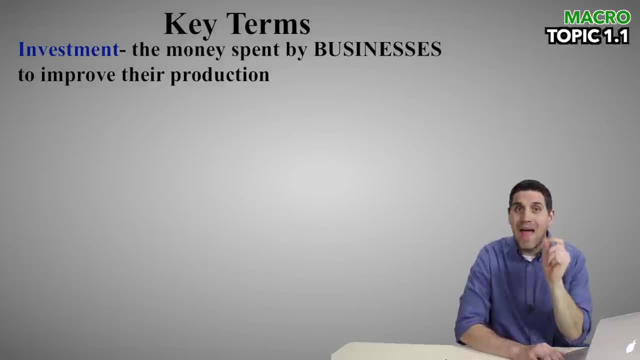 they're buying things to improve their business. Now I use the term. I use this term: capital. You're going to see that too, A lot of people think capital is money. No, no, no. There's actually two capital: goods which are made for direct consumption, like pizza, And there's capital. 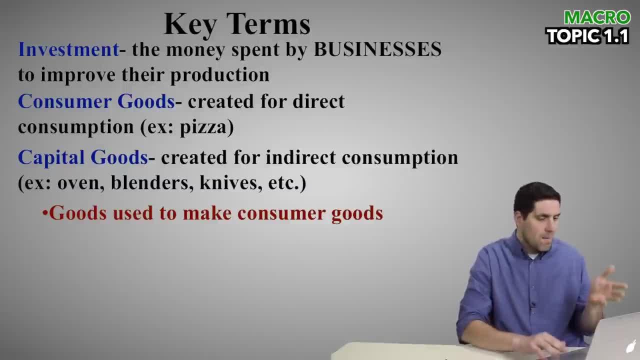 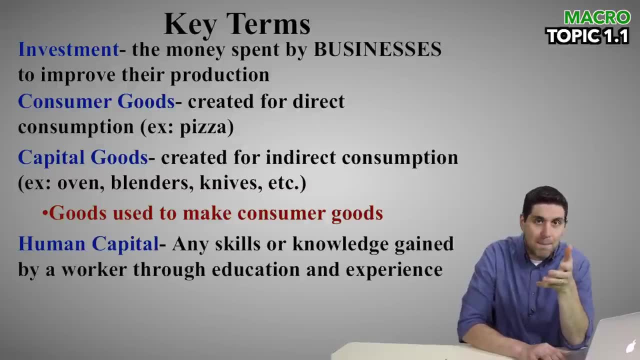 goods, Capital. goods are tools, machines to produce stuff. So blenders, ovens, knives, those are the things for a pizza company. that's their capital. Now, there's also something called human capital. Human capital is the knowledge and skills required to produce things. So, like a doctor, 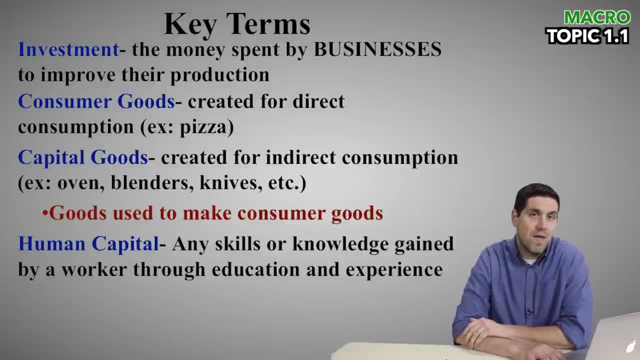 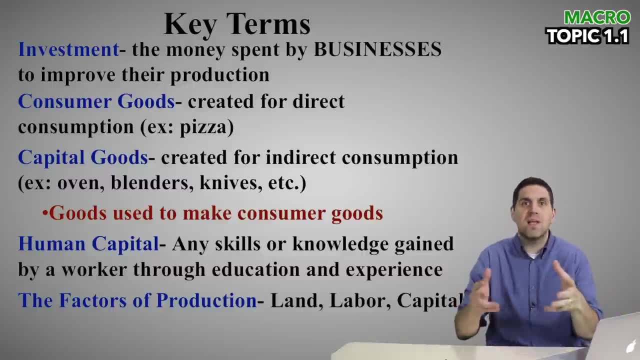 goes to school to get human capital, and you can improve those things over time. Now, another thing you're going to hear is something called the four factors of production. When you produce something, if you produce a computer, if you produce a table, if you produce a cell phone- there's 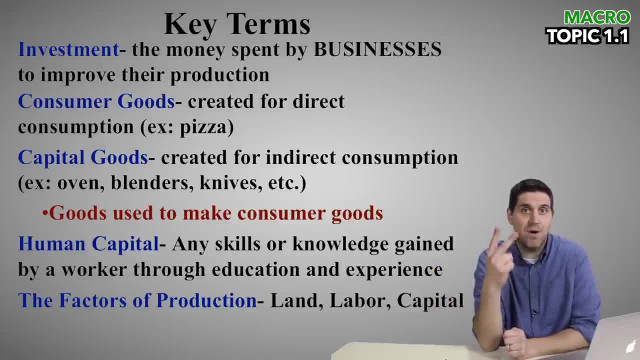 resources that go into it, And they can be categorized into four things: land, labor, capital and some people say entrepreneurship. So inside any product there's certain resources go into it. Who owns the resource determines what kind of economic system you have. Now let's look. 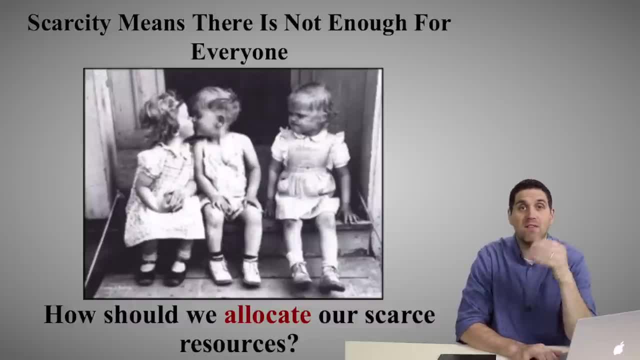 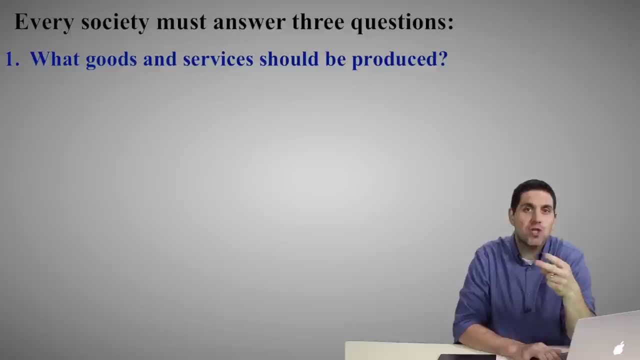 at the big picture. Scarcity means there's not enough for everyone, So we have to figure out the best way to allocate our scarce resources. Now, how we do that determines something called our economic system. There's three main economic questions every society has to answer. 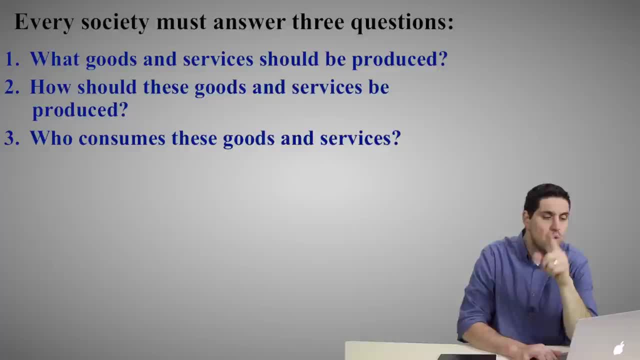 What goods and services should be produced, how it should be produced and who consumes those goods and services. So how do you figure this? how to run society? Well, basically, the idea is, if you answer these questions, the answers are all the government decides. 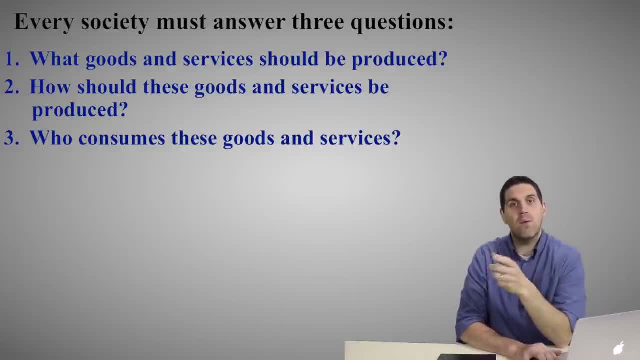 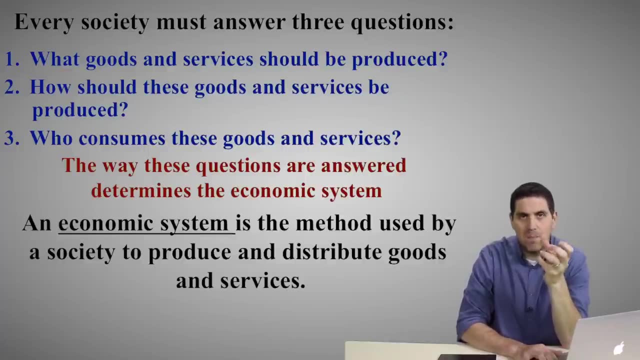 The government decides. That's one way to run society, And there's another way where individuals decide. So the way these questions are answered determines your economic system. It's the method society uses to produce and distribute goods and services. Now there's 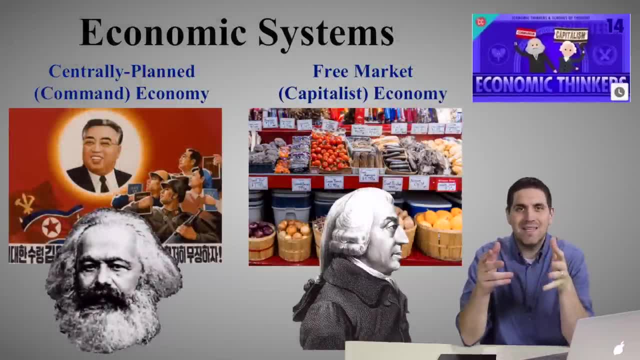 really just two main types we're going to talk about. We go into a lot more detail in other videos, But the idea is centrally planned and free market economies. The centrally planned economy is one where the government owns all the resources. It owns, basically the workers. 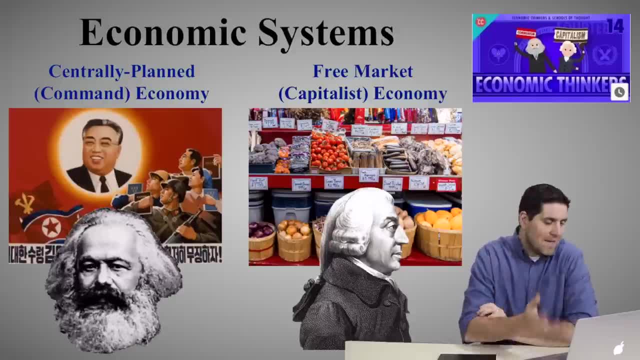 and tells them where they can work and what jobs they should have. The basic ideas came from the idea of Karl Marx, and there's a bunch of other people who pushed the idea of centrally planned economies. Now, free market or capitalist economies come from the idea of a guy named. 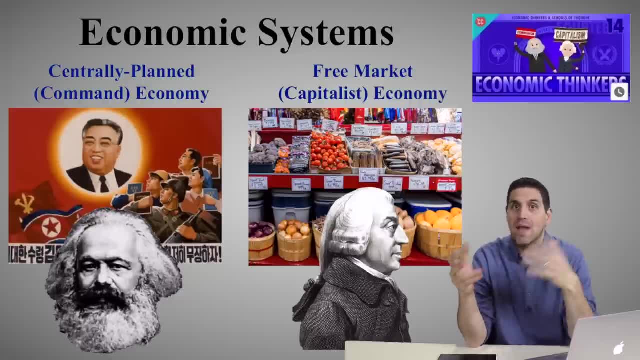 Adam Smith. He basically said: let individuals decide what to produce and how to produce it and who gets it. How does the market do it? Oh, that's called capitalism. Now your standard AP or college introductory course is going to talk about free market economies. They're going to focus. 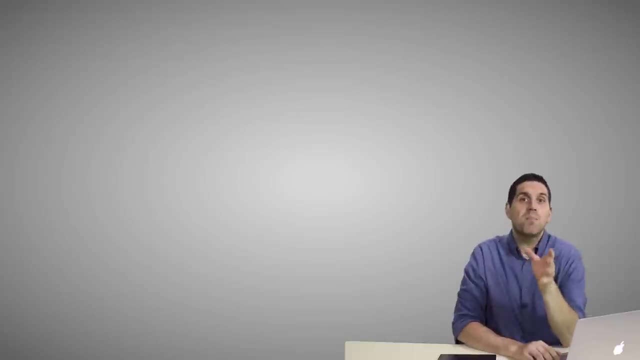 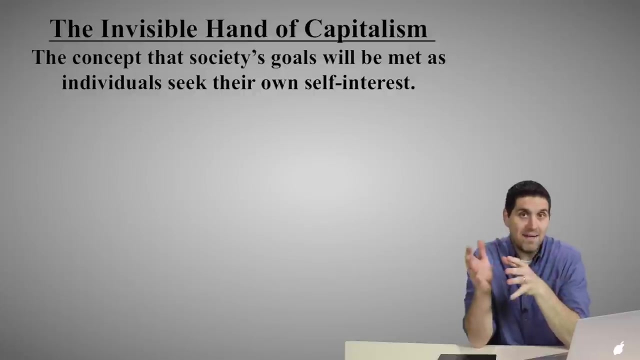 on those, because really that's what most of the world is doing. The most important concept in capitalism is the idea of the invisible hand. The invisible hand is the idea that society's goals will be met as individuals seek their own goals. So a business can't. 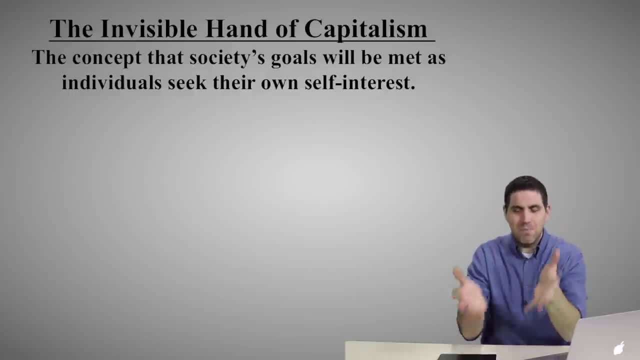 get rich and can't make money unless they do something that you want, Like if I produce cars, I got to make awesome cars. I got to make awesome computers, I got to make awesome phones. If I don't, then people aren't going to buy them, So they're going to make other people better off, And so society's. 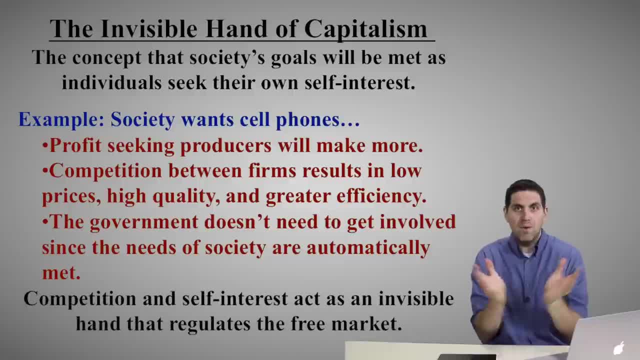 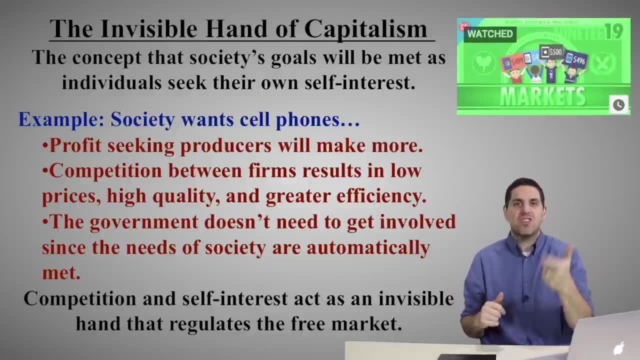 resources will go to the right place, based on what we want produced. Competition and self-interest regulate the free market system. Now there's all sorts of situations. this doesn't work with monopolies and externalities and other concepts you're going to learn in. 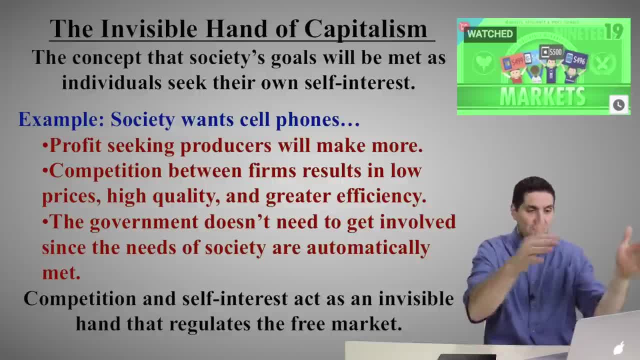 this course. But the idea of the invisible hand is the reason why this computer was not made by the government. That camera was not made by the government. A lot of the stuff around you was not made by the government. That's true, And that's not necessarily a bad thing. But we don't want the government. 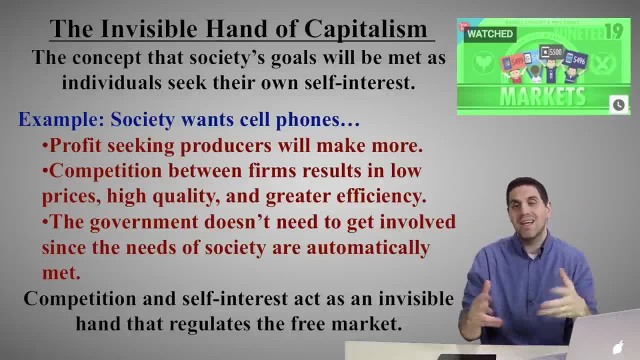 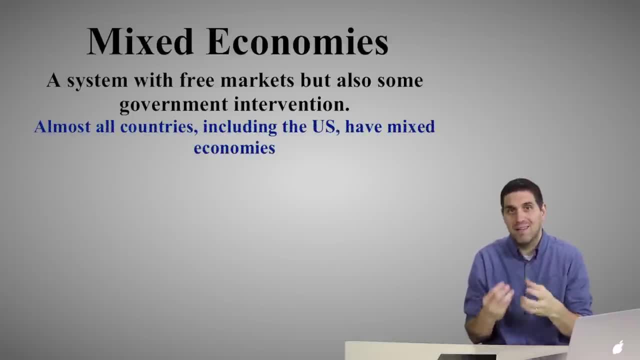 saying exactly what to produce and how much to produce, and who gets it. That system hasn't worked And that brings us to the idea of mixed economies. A mixed economy is a system that has both free market and centrally planned, like parts to it Some government involvement. 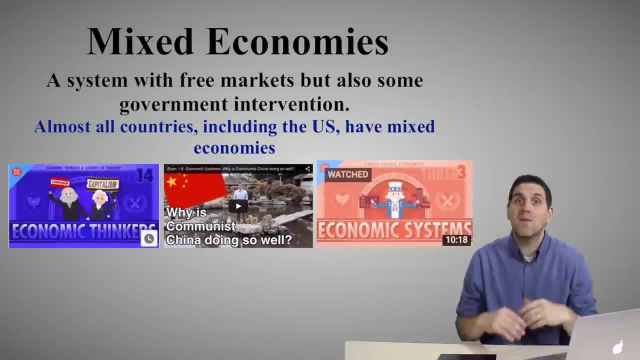 in different things. more government involvement in some countries than others, But if you want to learn more, go ahead and click on one of these. You've got economic thinkers and you've got economic system. I did those with the crash course people. There's also. 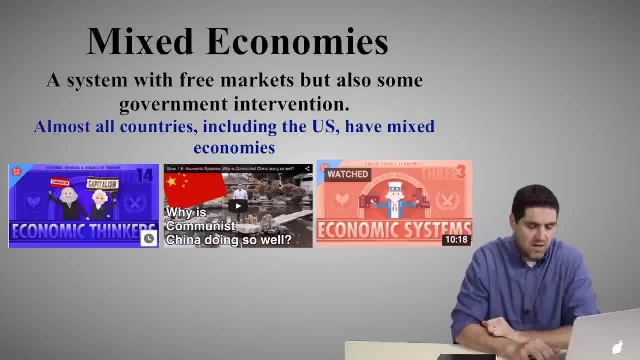 a video of me going to China, where there's Chinese lady check me out. It's pretty funny. Take a look. Anyways, let's move on. Now it's time for the key graph in this course, something called the production possibilities. 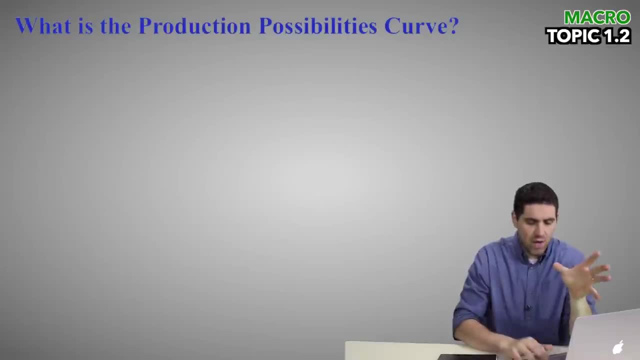 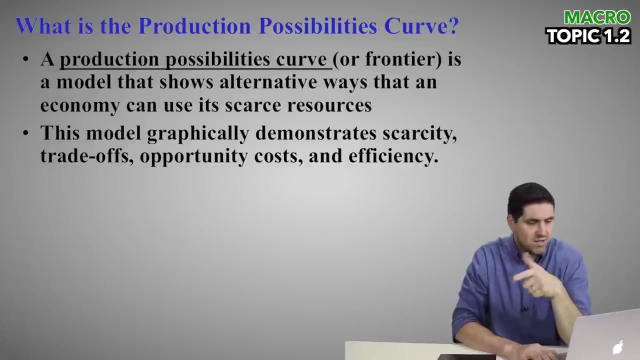 curve. Now your teacher might call it the production possibilities frontier. The point is it's all the same thing. It's basically a model that shows the alternative ways we can use our scarce resources. It's going to show trade offs, scarcity, opportunity, cost. 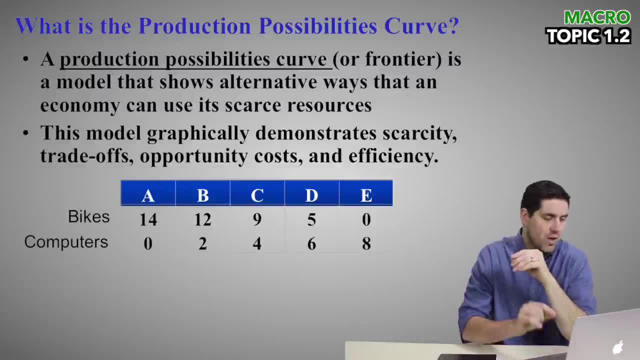 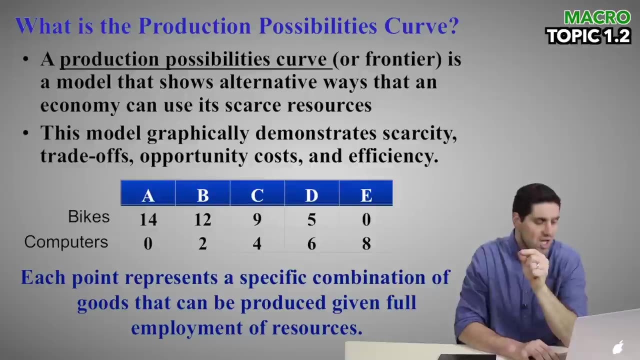 efficiency all on one graph. Now it starts off with a chart. This chart showing bikes and computers- A, B, C, D- is all different combinations, so we can produce all bikes and no computers. So if you actually plot this, you come up with a production possibilities curve Each. 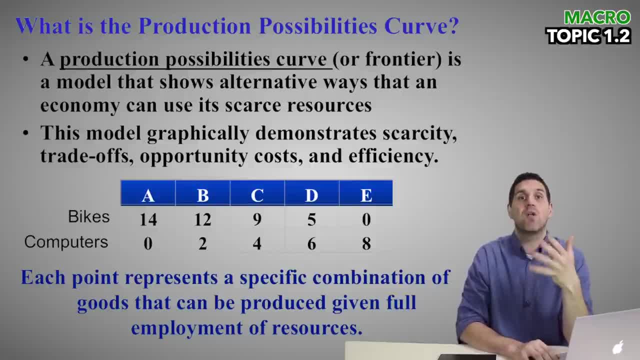 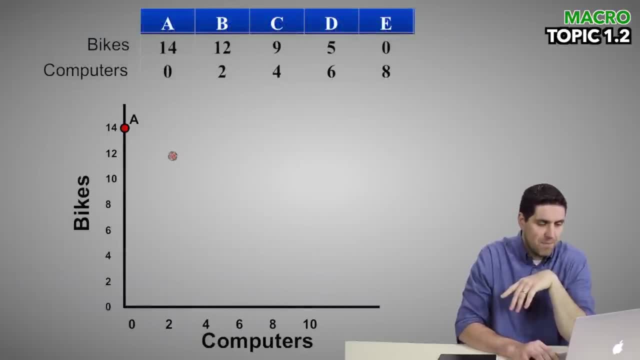 point represents a specific combination of the two goods we can produce at full employment using all of our resources. So if we take the chart, put it on a graph, it's going to look like this: You've got bikes, computers, and you plot the different points and you've 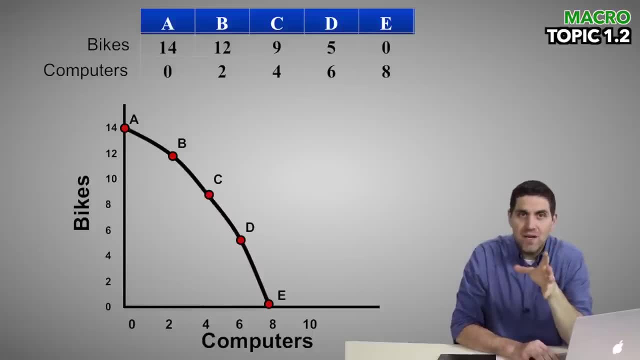 got boom right here. production possibilities curve. Now a couple things you need to know. First, any point inside the curve is the idea of inefficiency. If we're producing only two computers and two bikes, we're being inefficient with our resources. If we're producing any. 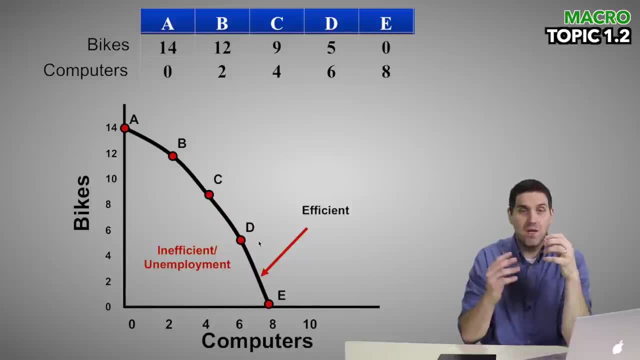 point on the curve, then we're actually producing what's efficient. We're producing using all of our resources, all of our workers, all of our factors of production to produce this stuff. And outside the curve you can't produce that quantity, There's just not enough. 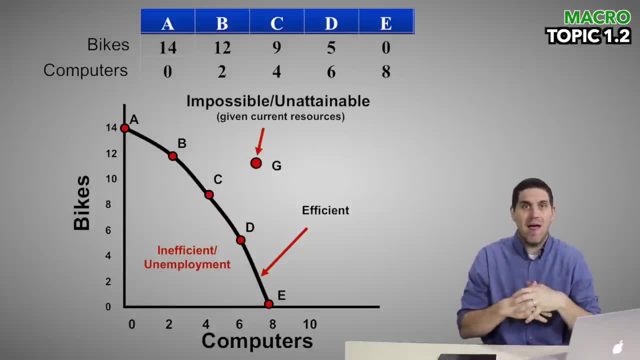 resources. So we could. if there was more technology and better resources, we could produce out there in the future, but for right now, for whatever reason, we cannot produce right here at point G. OK, there's a couple of different shapes to this graph And I want you to take a look. 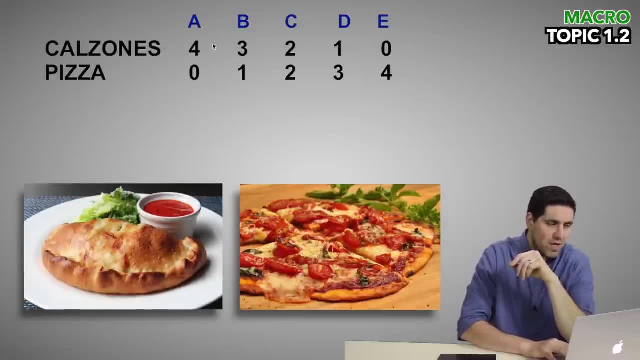 at it. calzones and pizzas. Notice: when you produce another pizza, you lose one calzone. When you produce another pizza, you lose another calzone. When you produce another pizza, you lose one more calzone. Now the opportunity cost here it's constant Every single time you produce a pizza. 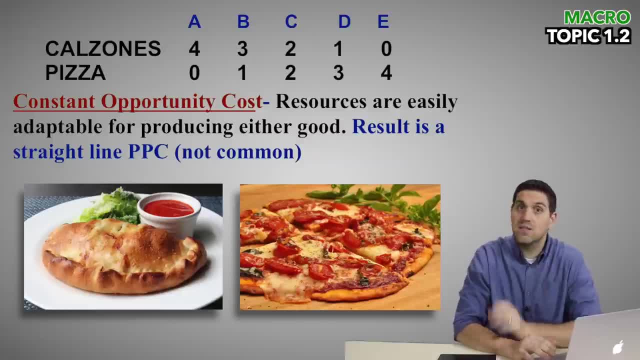 you lose one calzone. That's called constant opportunity cost and it shows you that resources between the two products are very similar. You can use resources for pizza, the same resources for producing the calzones. Now it's going to result in a production possibilities curve. that's. 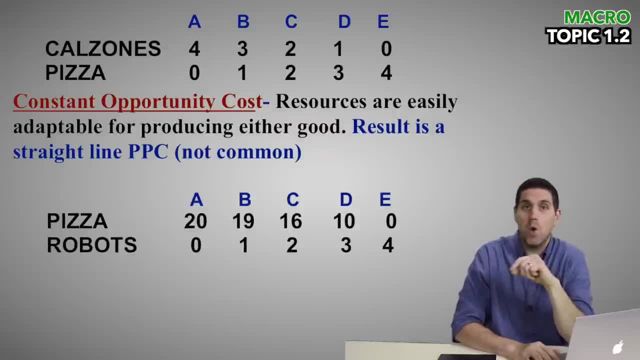 a straight line. Now let's look at a different scenario. Let's look at pizzas and robots Right here. when I produce the very first robot, I gain one robot, but I lose one pizza. When I go here, I gain one more robot, but now I lose three pizzas. Later on, I gain one robot and I lose. 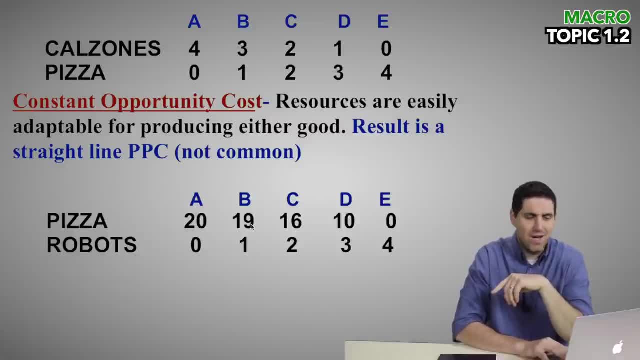 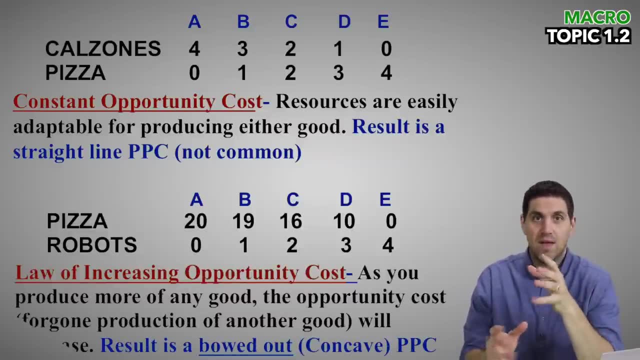 10 pizzas. Notice I lost only one pizza here and now I'm losing 10 pizzas. Something's going on and it's called the law of increasing opportunity cost. As you produce more of anything, the opportunity cost to produce. it's going to get bigger and bigger. 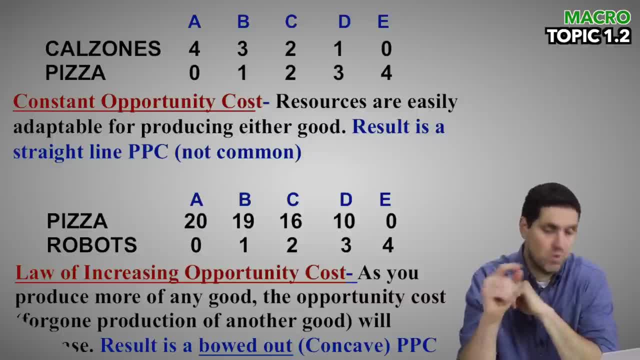 The reason why I'm using this law of increasing opportunity cost is because it's going to give me more resources. The reason why is because resources are not easily adaptable between the production of these two products: pizzas and robots. Let me explain why with an example. If 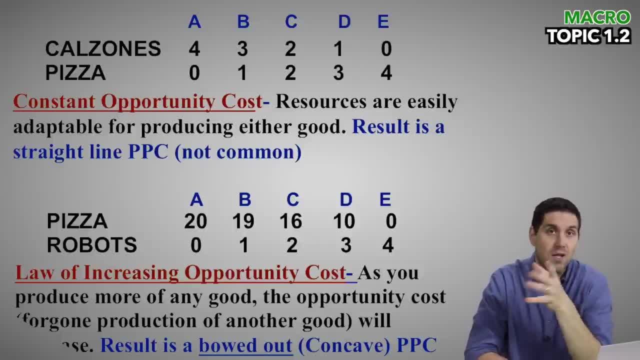 we're producing combination A, we're producing all pizzas. All workers, including workers that are better suited towards robots, are working at producing pizza. Now, when we move to combination B, we're moving out those scientists and those people who are good at making robots. We gain. 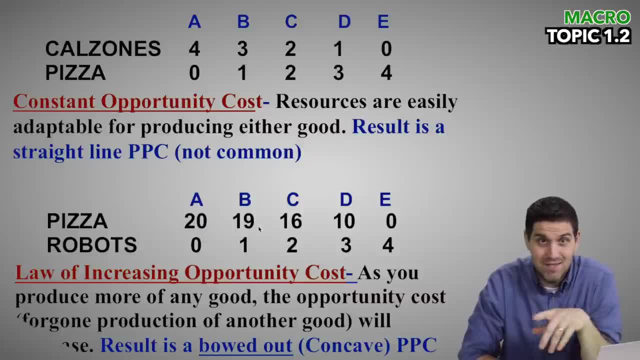 one robot and we don't lose very many pizzas because they're not particularly good at making pizzas anyways. Now if you keep doing that, you're going to keep moving resources away are out of producing pizzas towards robots, but eventually you'll start using the resources that. 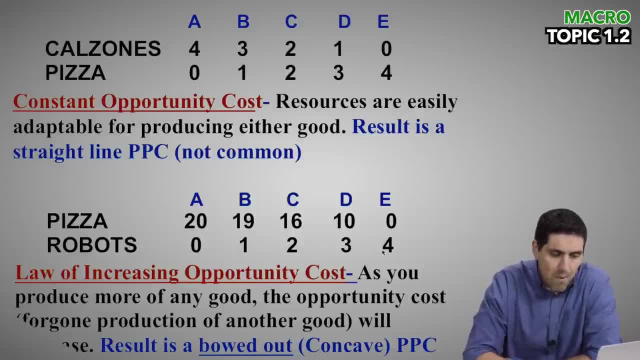 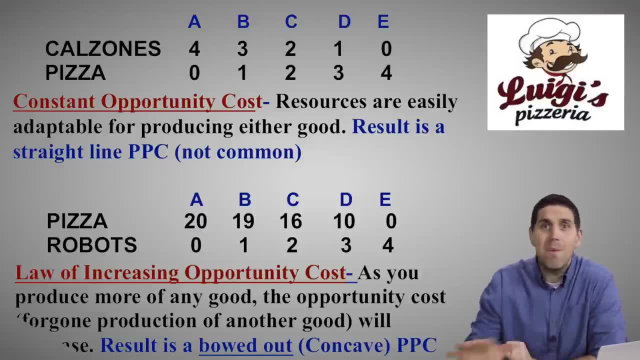 are better suited towards making pizza. For example, right here we get only one more robot, but we're moving away these pizza makers, who that's what their job is- right, Luigi, working in the back of the pizza restaurant. He's way better at making pizzas than he is robots, So 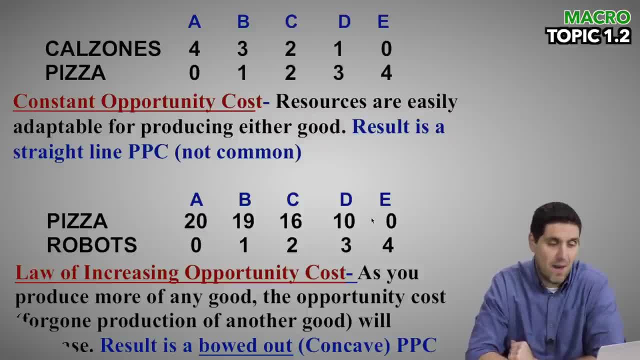 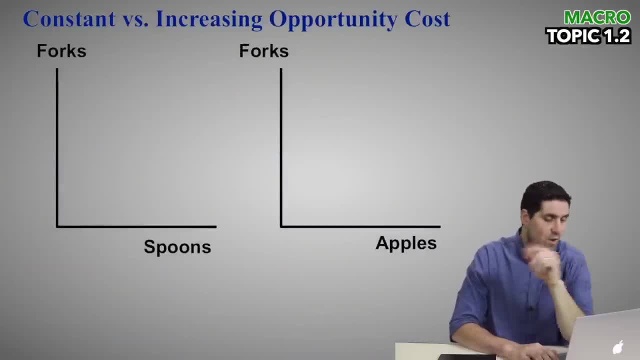 the opportunity cost is super high. Remember, it's 10 pizzas we have to give up moving from D to E. Again, this is called increasing opportunity cost. Let's see if you understand it with another example. We've got forks and spoons. 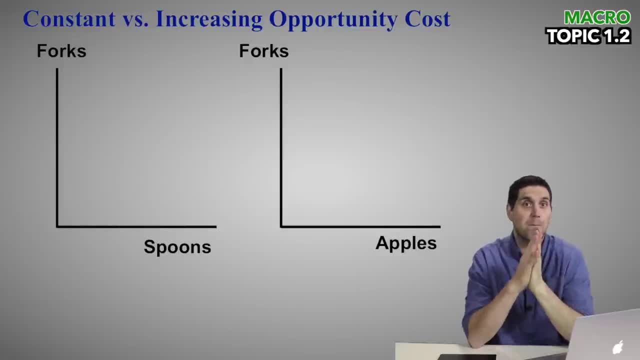 forks and apples, Which one of these is a straight line and which one is a boat out curve. Well, right here: Forks and spoons- straight line, that's constant opportunity cost, And the boat out forks and apples, that's increasing opportunity cost. The idea here is: you produce more and more. 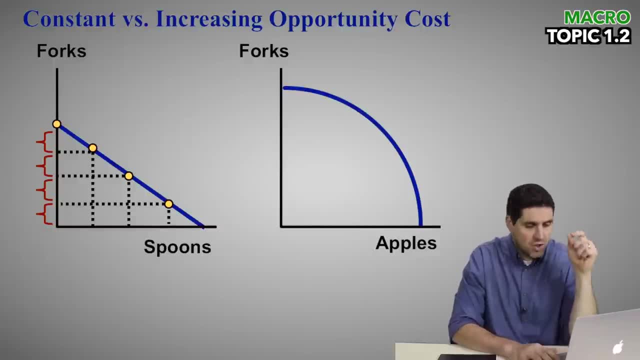 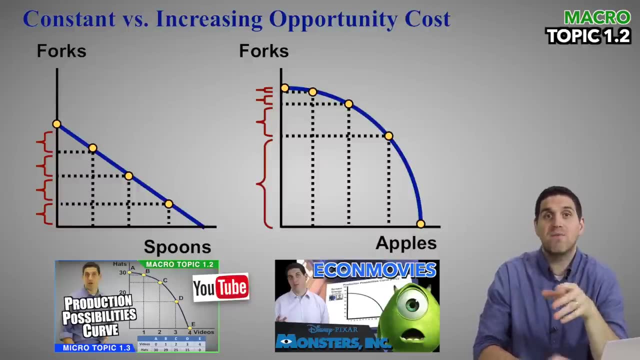 spoons, you're going to give up the same amount of forks each time, But as you produce more and more apples, you're going to have a little bit of forks and more forks, and more forks and a whole lot of forks. Now I've made a bunch of videos explaining this concept. In fact, I've made 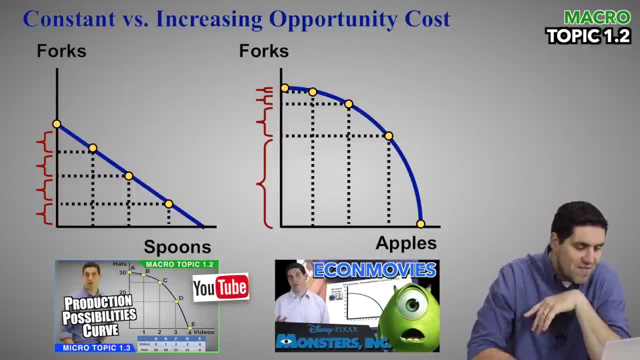 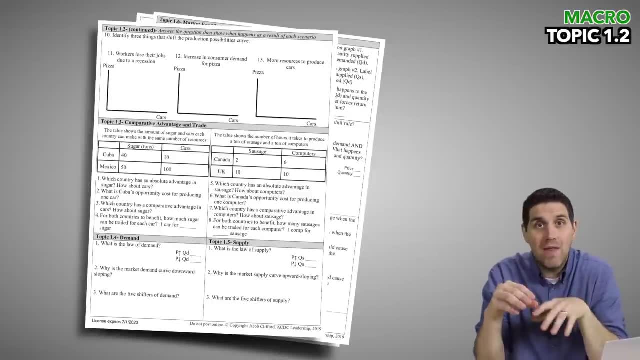 something called econ movies. If you haven't seen them, take a look. But I've explained it in this video. I'm not going to talk about shifting the production possibilities curve in this video, But there is some practice questions on your packet. Make sure to try those because it's pretty. 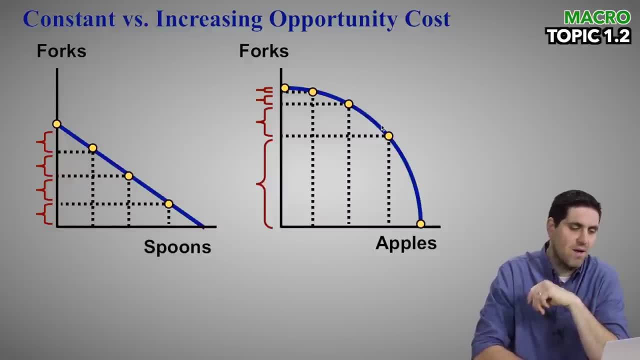 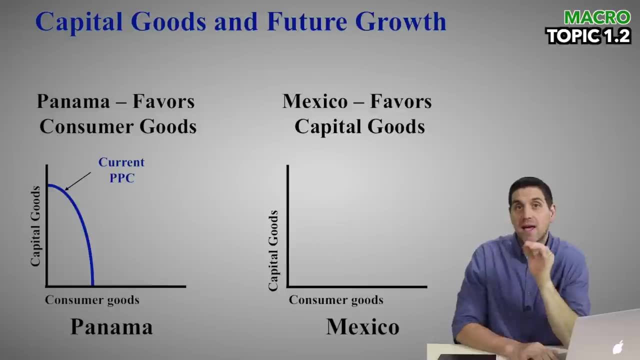 self-explanatory. If, for whatever reasons, we have new technology, this entire curve can shift outward. We can get more forks and more apples. One of the things I do want to cover is the idea of growth in the future. So take a look at two different countries. We've got Panama over here. 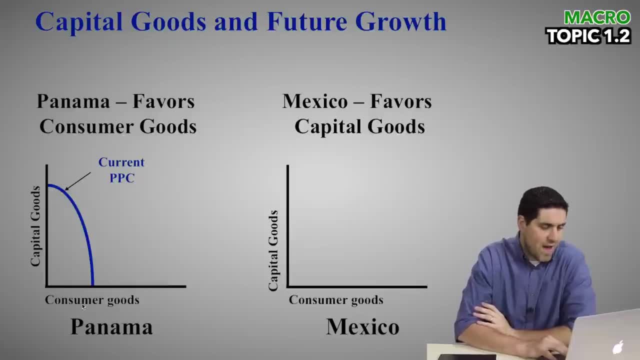 We've got Mexico over here. Let's say here's the production possibilities curve for Panama. They can produce consumer goods and capital goods. Let's say they're producing a certain combination which is producing a whole lot of consumer goods. Now their future growth curve. I'll put right. 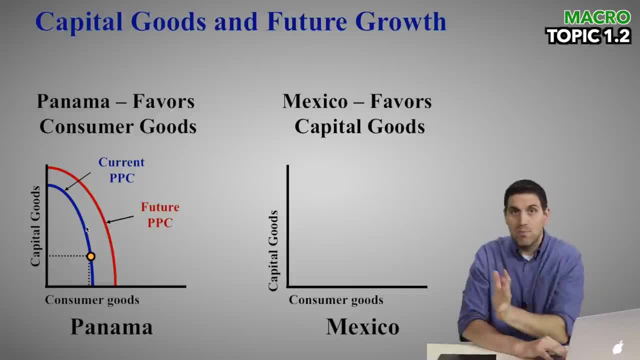 here is out here. So they'll have growth over time. They'll be able to produce more in the long run. But over on this side, take a look. Let's put another country. There's Mexico, and they're producing this combination: Less consumer goods, which sucks. They're getting less bananas and 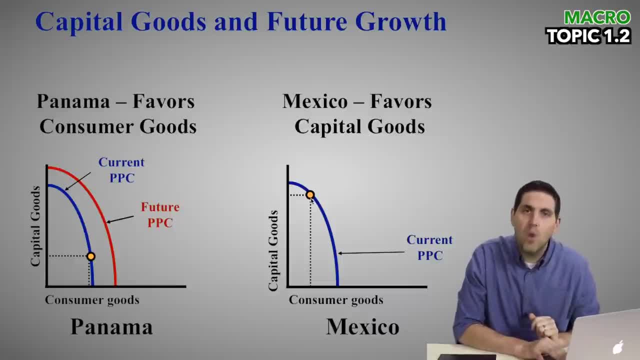 clothes and stuff like that, But they are getting a whole lot more capital goods. The question is: what's the future curve going to look like for Mexico? Is it going to be the same distance out as Panama? Is it going to be farther out? Is it going to be farther out? Is it going to be? 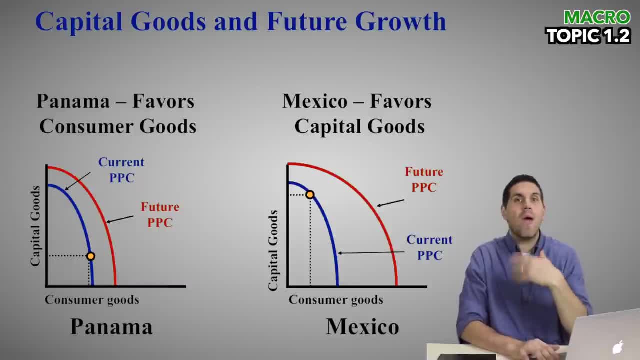 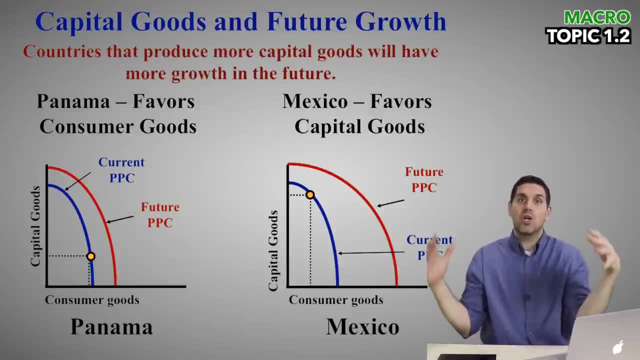 less growth. Well, it's right here: There's going to be way more growth. Why? Because capital is a resource. The more capital you produce, the more production you can do in the future. because capital is a shifter of the curve. You can get more output by producing more capital. So I know. 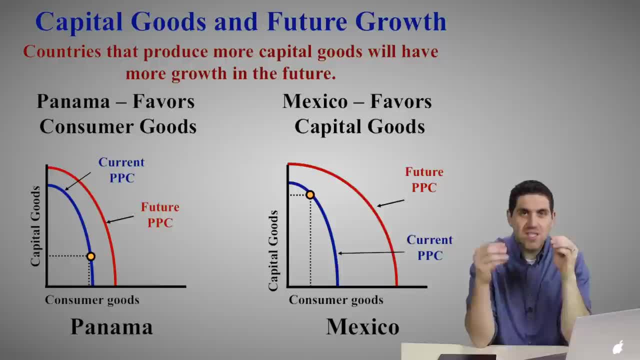 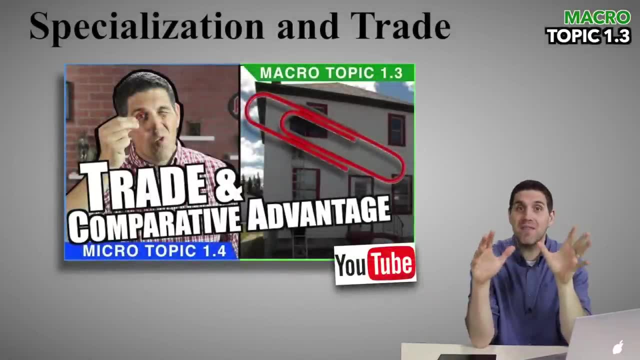 it seems like I'm rushing through this stuff and I'm not trying to, but just trust me, this first unit, the beginning stuff, is really easy. That's why I'm going really fast. Trust me, you're going to get it. It's easy. Now I'm going to slow down. This is something that's a lot trickier. It's. 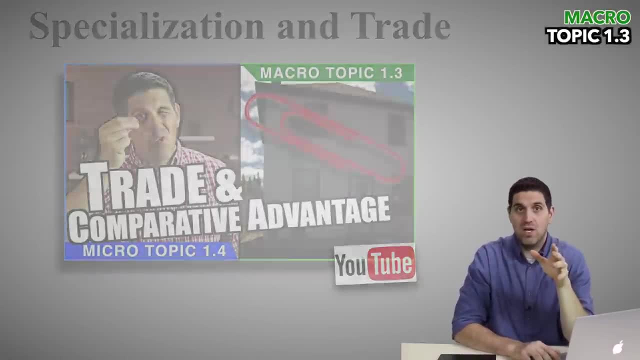 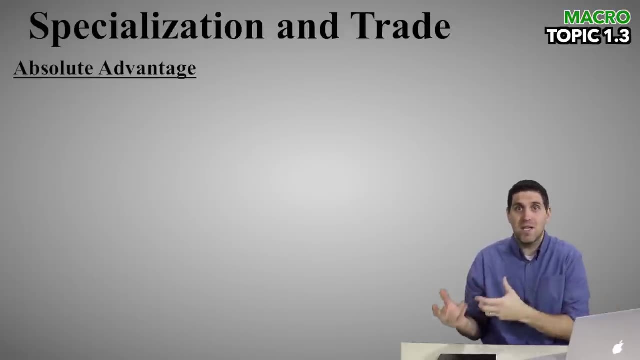 called specialization in trade. It's called specialization in trade. It's called specialization in trade. It's this idea of comparative advantage. It starts off easy, The idea of absolute advantage. People are sometimes better at producing than other people, So some people can produce. 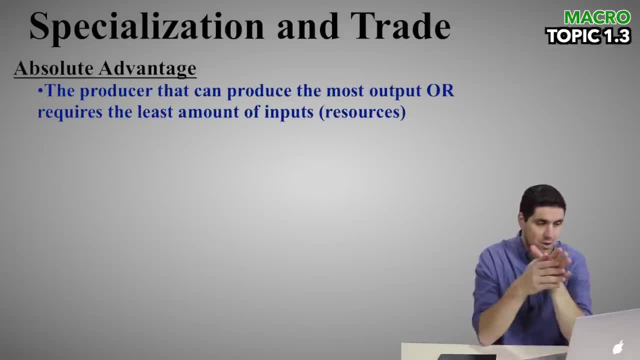 things better than other people. This is the idea of absolute advantage. They can produce more output or they can use fewer resources to produce the same output as some other person. They're just better at making things. Now, the United States probably has an absolute advantage in the 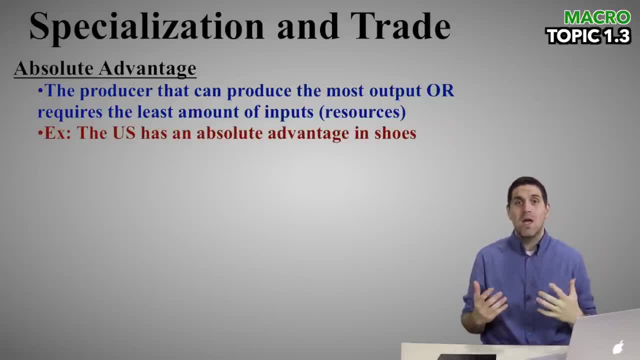 production of shoes And we could probably produce a boatload of shoes if we wanted to, because we could And we're just a very large, powerful productive country, But we don't produce shoes. We could- We probably could- produce the most in the entire world. 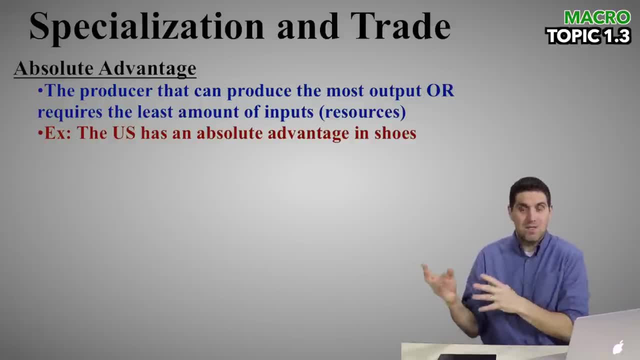 but we don't. We specialize in other things that we produce. instead, We let other countries specialize in shoes. Now, that's the idea of comparative advantage, Comparative advantage, the idea of having the production, having a lower opportunity cost, So I can produce this. 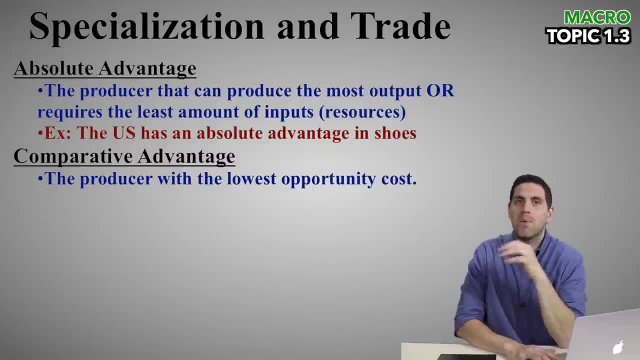 at a lower opportunity cost than somebody else. The United States produces very few shoes, but we produce a whole lot of things like airplanes or CGI movies, right Movies like Pixar movies. We produce a lot of computer movies because that's what we're good at And we have a lower 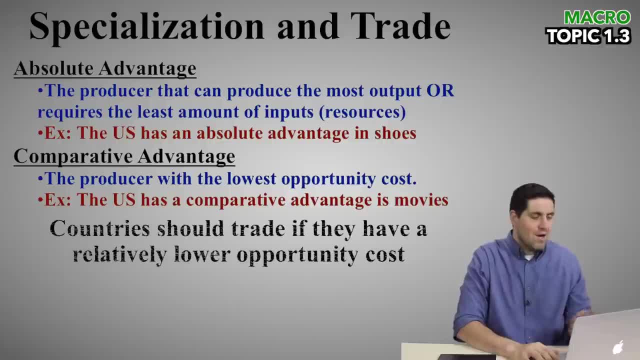 opportunity cost than another country who can't produce those things. The idea here is that countries should specialize in trade when they have a comparative advantage. If you're better at producing something than I am, and I'm not as good as that producing that thing and I'll. 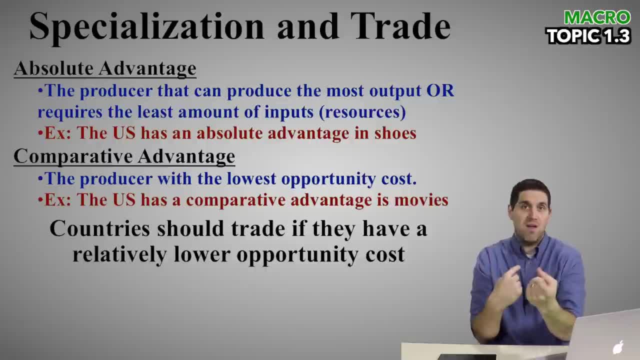 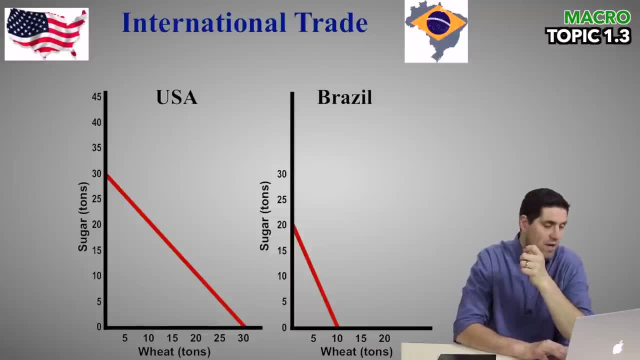 specialize in the thing that I'm really good at. we both can trade and we can both benefit, right, So I'll trade you the movies, you trade me the shoes. we both walk away happier. This is a production possibilities curve. It shows you how much sugar and wheat the US can produce and how 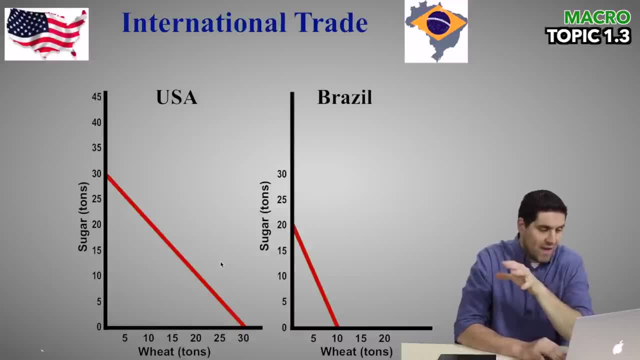 much Brazil can produce. Now, first question: which country has an absolute advantage in the production of sugar? Well, the United States. They can produce 30 tons, and Brazil can only produce 20 tons. So the United States can produce more sugar. Now, who has an absolute advantage in the 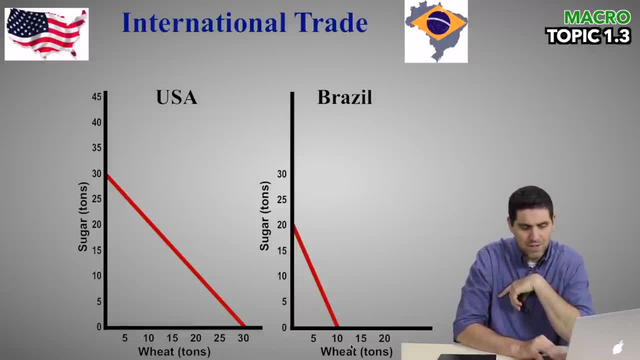 production of wheat. Well, the United States, They produce 30, and Brazil can only produce 10.. So you can see, the United States has an absolute advantage in both. Now people assume that if the United States can produce more of both, we should produce both. But we don't. This is the idea of 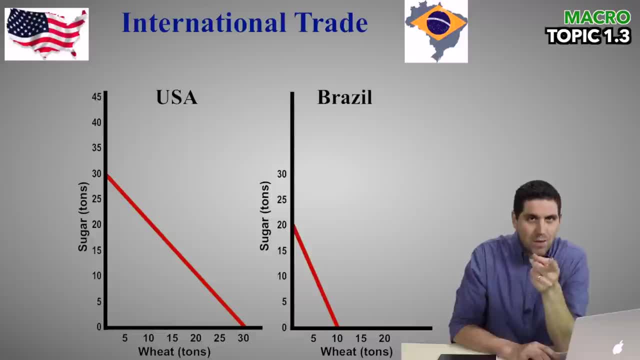 international trade and comparative advantage. So I'm going to work backwards here, but stay with me. Let's say the United States specializes in wheat and Brazil specializes in producing the sugar, and they trade one wheat for one and a half sugar. I'll explain how I got that. 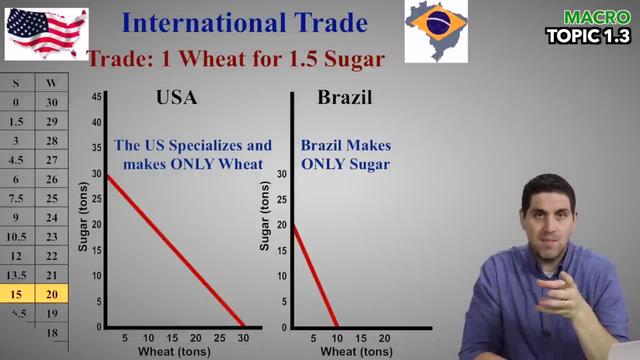 number later. but just stay with me. Take a look at this. new production possibilities curve. This is the new numbers based on the trade. If the United States produces all wheat, then they can produce 30 wheat, right. They're down here, they're producing 30 wheat and they trade one of their wheat and they get one and a half. 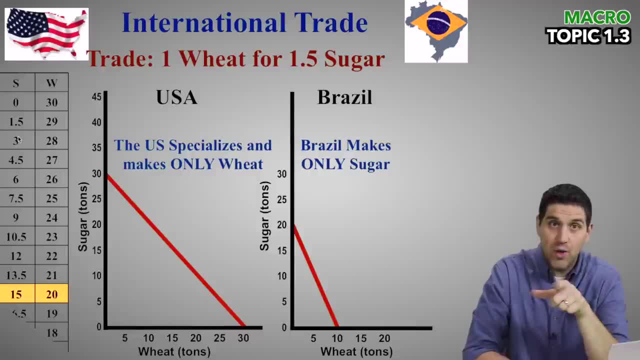 sugar. They trade another one wheat. they get another one and a half sugar With the trade. Look down at this number: 20 wheat and 15 sugar. 20 wheat, it's right here. 15 sugar is outside the curve. 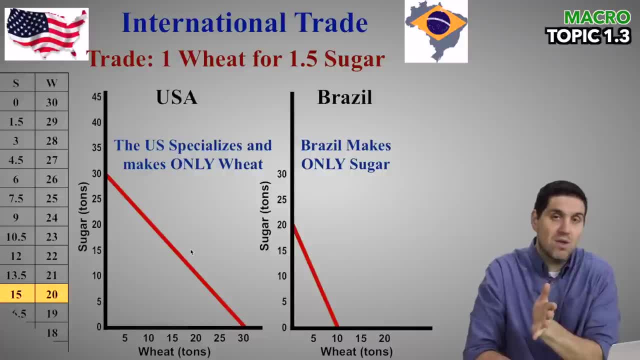 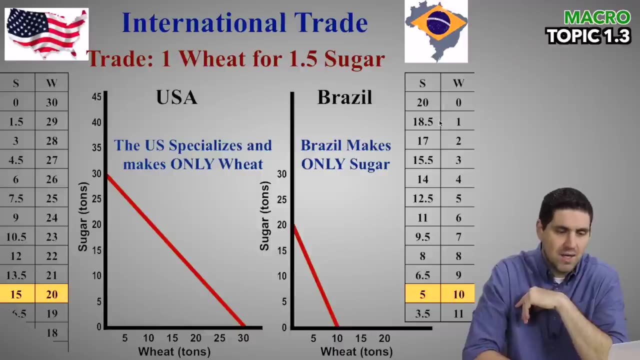 They're producing. in fact, they're consuming, not producing. they're consuming outside the curve by trading, Because they're getting that sugar at a lower opportunity cost than if they produce it themselves. Look at Brazil. If Brazil produced all sugar, they produced 20 sugar. they can trade one and a half sugar to get one wheat. 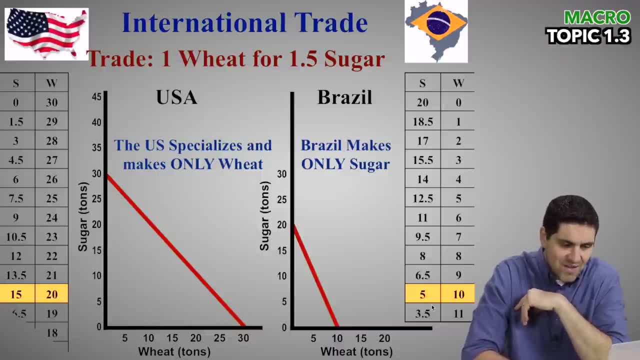 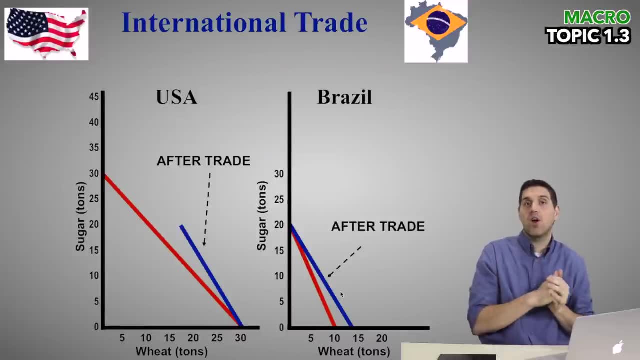 Another one and a half sugar for one wheat. Another one and a half sugar. Look at this number here. Five and ten. Five sugar is here. ten wheat is out here For both countries. after trade their curves can shift outward and they can consume more than if they could produce on their own. 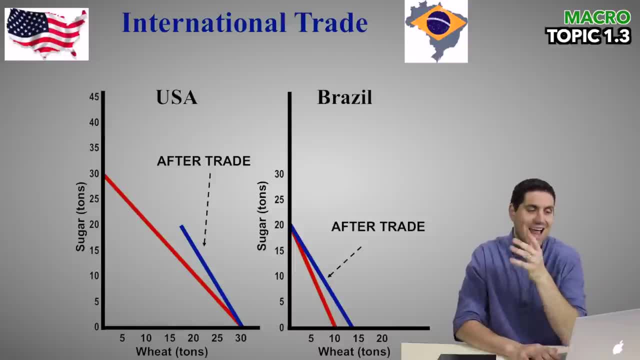 Right, That's the idea of the benefits of trade. Now the question is: how did I get those numbers? This is the tricky part, What you gotta do when you do these questions. first, you gotta convert the graphs into a chart. 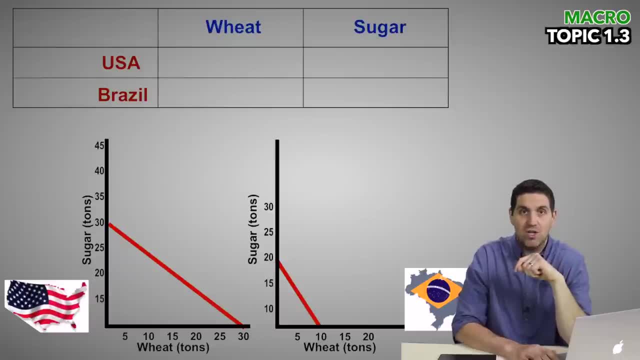 So I've got the countries US and Brazil On the top. I've got wheat, I've got sugar. Now I just plug in the numbers. The United States can produce 30 wheat or 30 sugar. Brazil can produce 10 wheat or 20 sugar. 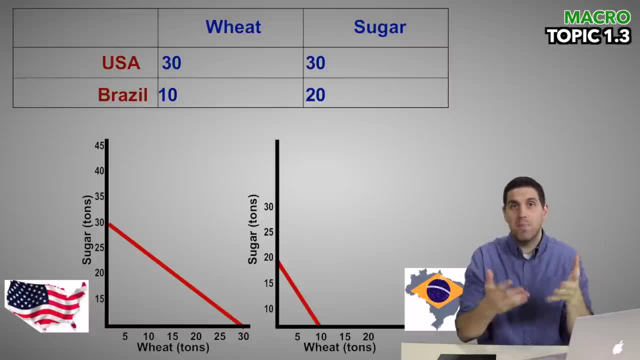 So absolute advantage is really easy to spot. It's just whichever country can produce more in this case. So the United States can produce more wheat. They have an absolute advantage in the production of wheat and in sugar. Now time to calculate comparative advantage. 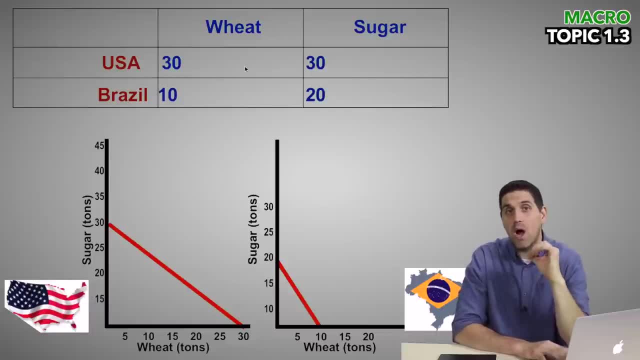 To figure out the comparative advantage, you gotta figure out who has a lower opportunity cost. So you have to calculate what's called the per unit opportunity cost for each country. Now it starts out pretty easy. By the way, the way I set it up is how I would do it with my students. 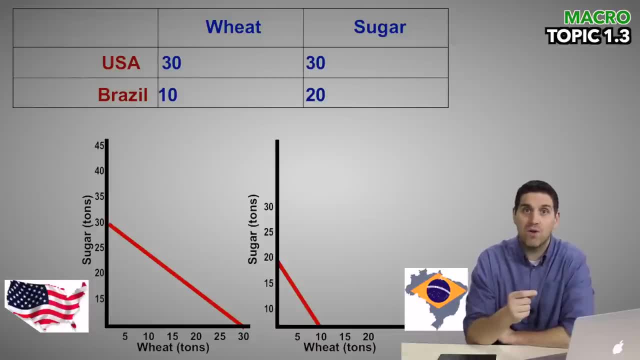 I would set up the chart, draw it out every single time like this and practice this over and over again. Your review packet has several practice questions, but don't do them yet. Wait until I cover this first, And I'm also gonna give you a trick. so keep watching. 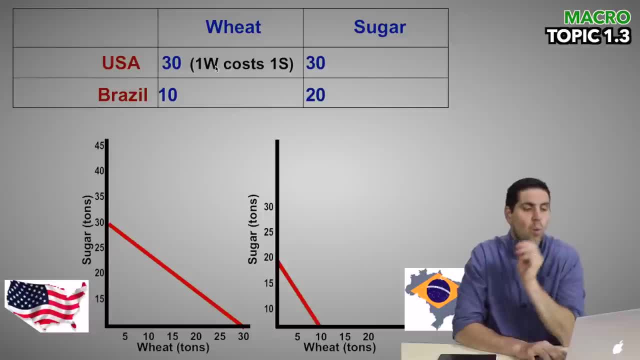 For the US, one wheat costs one sugar. If they produce one wheat, they're giving up one sugar. That's their opportunity cost. For the US, one sugar costs one wheat. That's an easy one. Now here's my question For Brazil, how much does each one wheat cost? 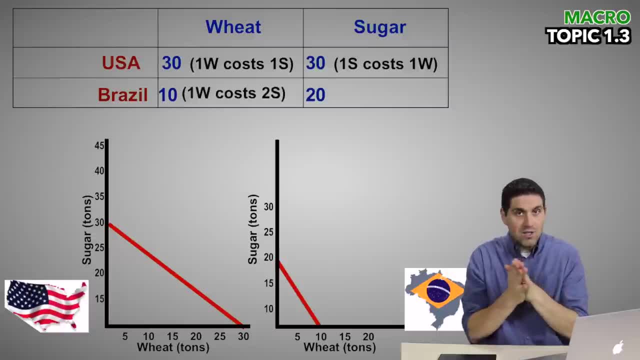 Well, that right answer is two. One wheat costs two sugar. Two sugars they could have produced, but they can't produce it when they're producing wheat. And on the other side, each one of the sugar is the reciprocal. It's one half. 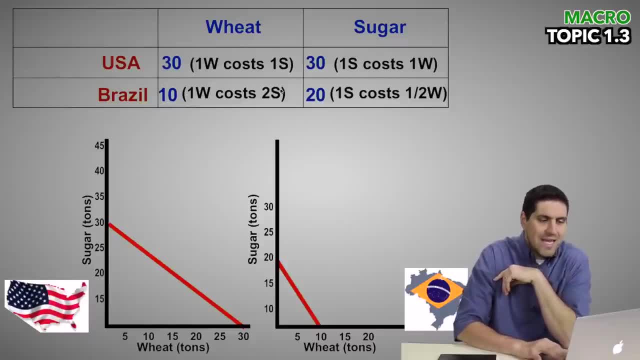 So if they produce twenty sugar and they could be producing ten wheat, well, each one of the sugar costs one half a wheat They gave up. Now that we have this, we can figure out the comparative advantage, because we can find out who has a lower opportunity cost. 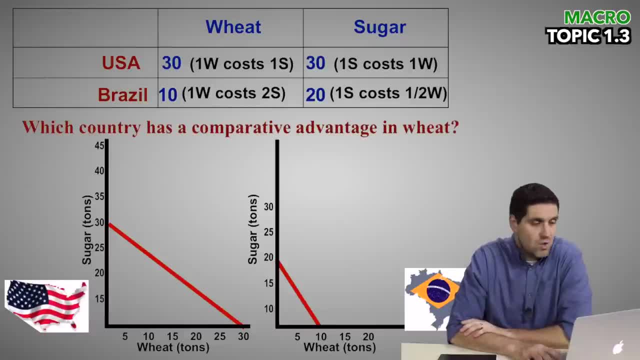 So which country should be producing the wheat? Who has a comparative advantage in wheat? Well, the United States. They have a lower opportunity cost and it only costs them one sugar compared to Brazil that costs them two sugars. So they have a lower opportunity cost. 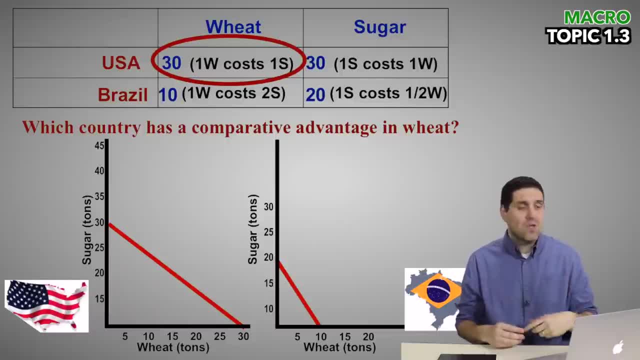 When they write these questions. you can't have a comparative advantage for both. So if you see a test question and you find out that the US has a comparative advantage in wheat, you're done. You know for a fact that Brazil has the comparative advantage in sugar. 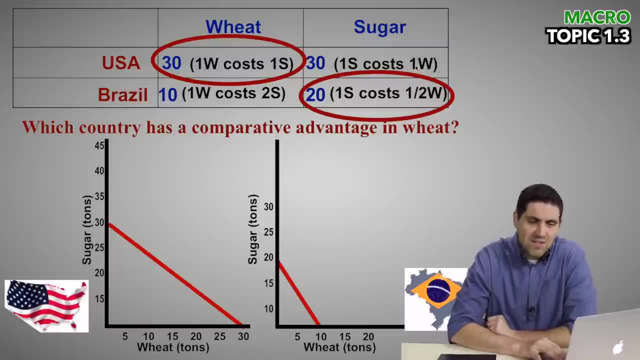 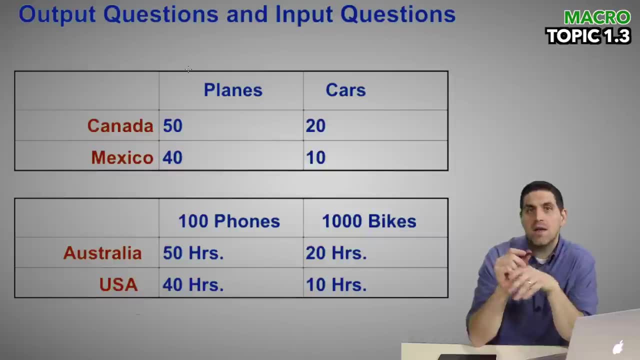 But it'll always work out that way. But look at the numbers. It makes sense too. One half is less than one. The point is to figure out comparative advantage. you've got to calculate something called per unit opportunity cost. Now there's two different types of questions. 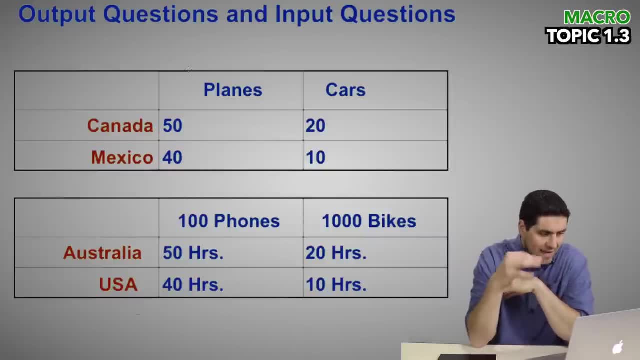 There's output questions and there's input questions. So for this one we've got Canada, Mexico. This is number of planes They can produce right here And this is the cars they can produce. So planes and cars, This is going to be an output question. 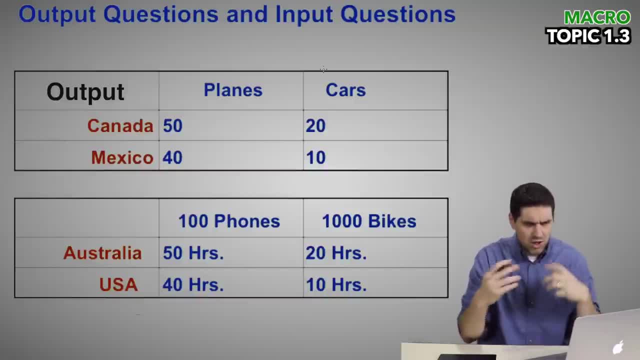 Now on a test question, they would give you more information. They'd say: this is number of planes and cars that Canada and Mexico can produce. But I'm just setting it up. That's the idea of an output question. Now, which country, real quick, has an absolute advantage in the production of planes? 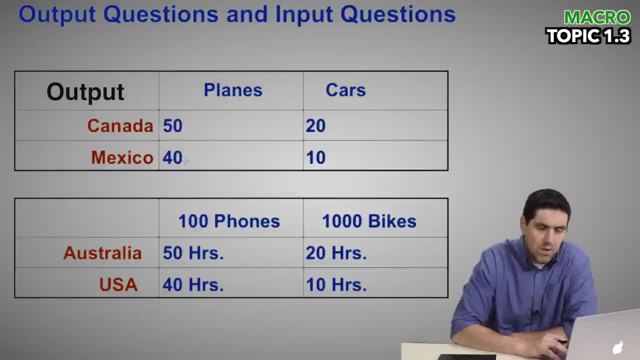 Well, Canada, They can produce more planes than Mexico. Which country has an absolute advantage in production of cars? Yeah, Canada, They can produce 20, and Mexico can only produce 10.. So Canada has an absolute advantage in both Good. 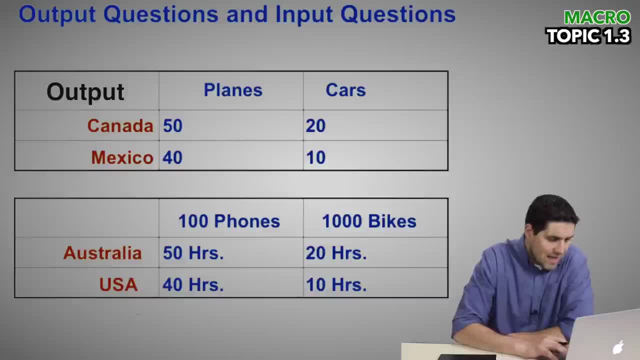 Very true. Now let's go look down here. This next one is the idea of Australia, US. This is number of phones If they produce 100 phones. this is if they produce 1,000 bikes. This is number of hours it takes to produce those 100 phones. 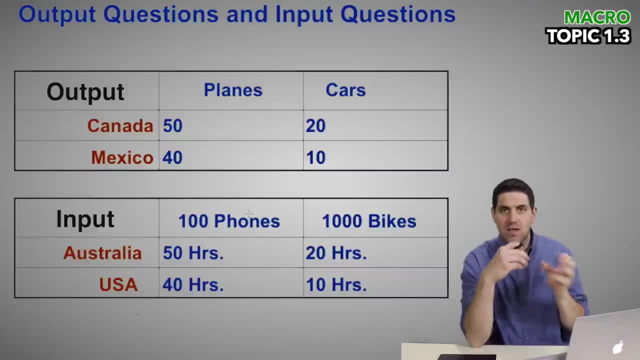 Now this is called an input question because the resource is what's variable here? So 50 hours to produce 100 phones, This one, US, takes 40 hours to produce 100 phones, And over here, Australia takes 20 hours to produce 1,000 bikes. 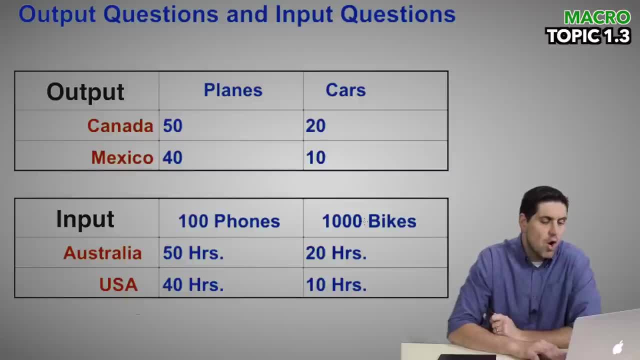 US takes 10 hours to produce those 1,000 bikes. Now the question is: who has an absolute advantage in the production of phones? The answer is the US. Notice: now you're looking for a smaller number because we're looking for hours. 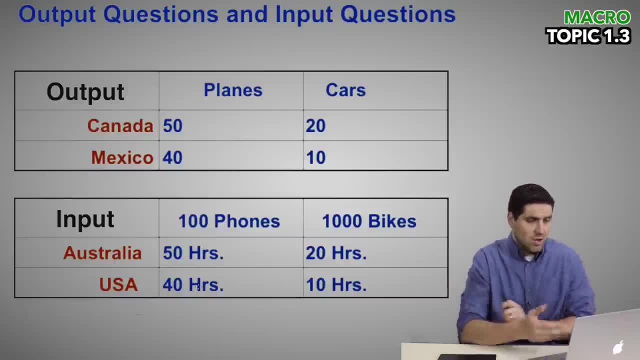 It's better to use fewer resources, In this case fewer hours to produce the phones. And over here, who has an absolute advantage in the production of bikes? Well, the US. They take fewer hours. Notice, the numbers are exactly the same. 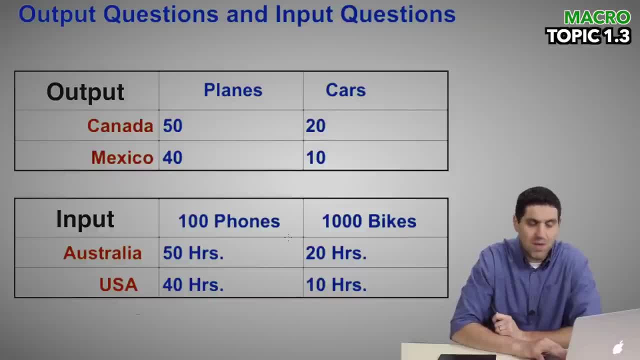 They're exactly the same numbers: 50-40, 20-10, 50-40, 20-10.. What matters is what the question's asking. If it's an input question, then we're looking at hours, Or if an output question, then we're looking at the number of things they're producing. 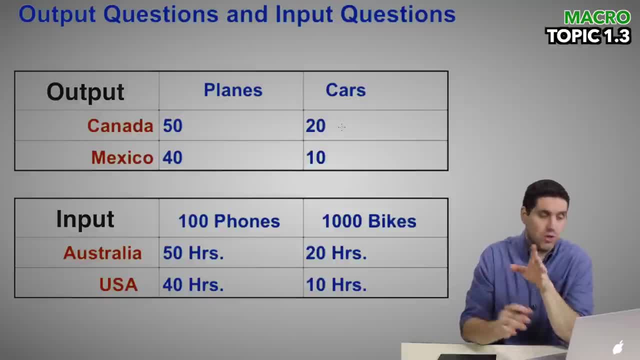 the stuff they're actually making. Now you can figure this question out by doing what I showed you earlier: Calculating the per-unit opportunity cost for Canada. So in this case it would be one plain cost. I'll put equal signs for cost. 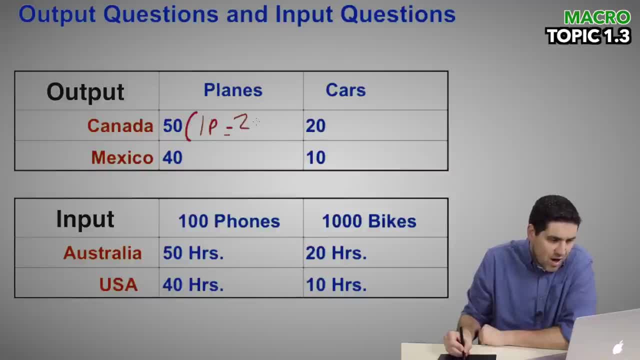 A certain number of cars given up. In this case it would be two-fifths of a car given up right Now. you could do that, but it's really time-consuming and some students get uncomfortable. It becomes difficult for them. 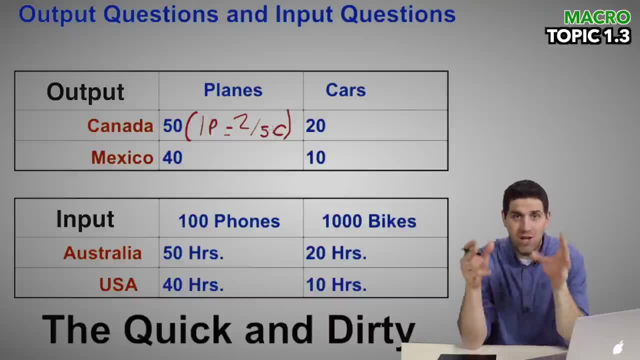 So here's a trick. It's called the quick and dirty. Now, the reason why it's called the quick and dirty? because it is super quick but it's dirty. It's so academically dirty, It's just, it's not cheating. 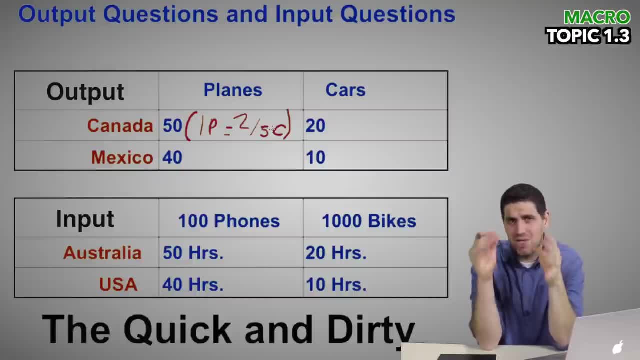 It's just like you're not going to learn anything. You just it's just a trick that's going to work every single time. And all the people who didn't watch the video up to this point, well, they missed out because 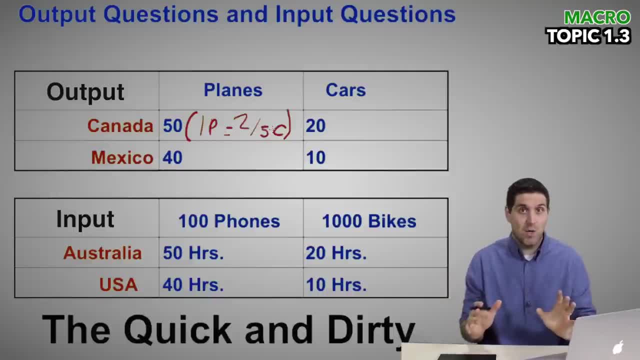 you're going to get the quick and dirty, Go ahead and tell all your friends about it. Mr Clifford did the quick and dirty with me. It was exciting. First, you understand the idea that there's only two possible outcomes. that's going to. 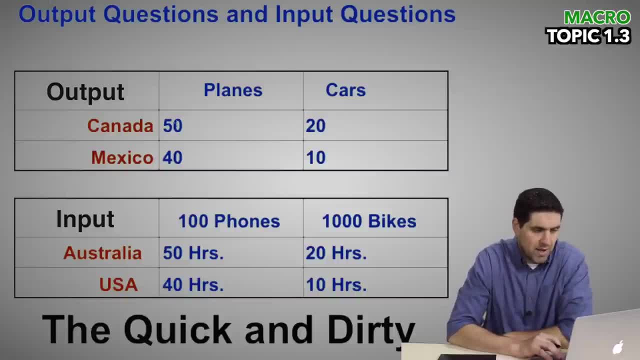 happen here, The comparative advantage: Canada should be producing the planes and Mexico would produce the cars, right. So it would be this situation, right here. It would be this. I'm going to draw a diagonal representing Canada would be producing planes and then 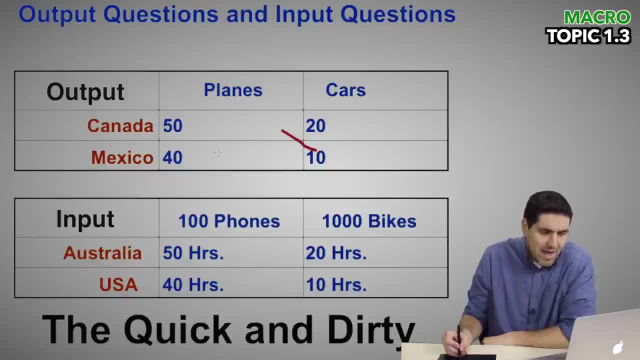 Mexico cars. Or the other option is Mexico is going to be producing the planes and Canada is going to the cars. So this other is the other possibility. Remember you can't have a comparative advantage in both products. They can't have a comparative advantage producing both. 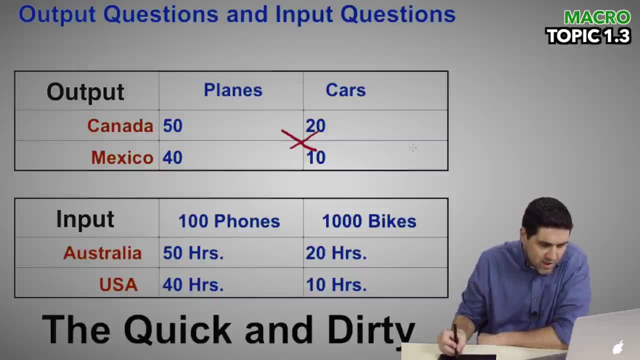 So here's the quick and dirty. So 50 times 10 gives you a certain total number of things produced, which would be 50 times 10.. Or the other one is 40 times 20.. 40 times 20 is 800.. 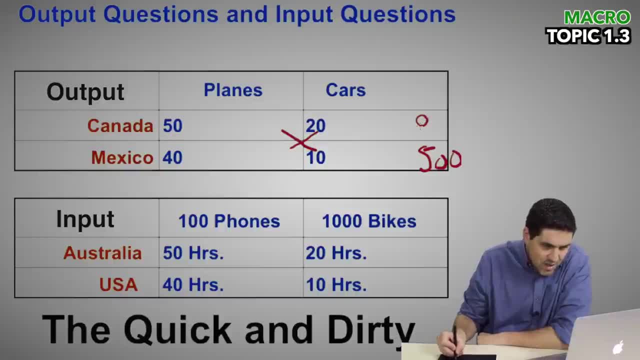 Now, since 800 is more than 500, that means that is the right answer. Bam, Quick and dirty, No doubt about it. Guaranteed, You can do all the other calculations if you want. Mexico is going to be producing the planes and Canada is going to be producing the cars. 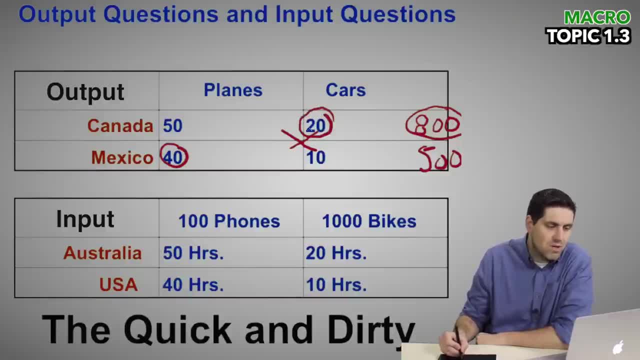 Right Again. here's how I got it: I multiplied the possible outcomes. It's either this or this The one that gave me the most. because that's what I'm going to do: I'm going to multiply the possible outcomes. 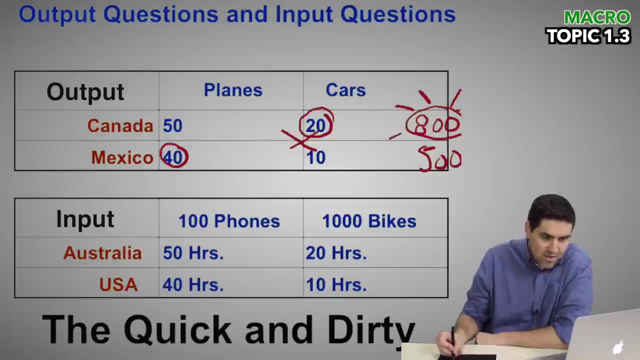 I'm going to multiply the possible outcomes. I'm going to multiply the possible outcomes. That's what I want. I want the most stuff. Right, That means it has a comparative advantage. Right, That's the idea of getting comparative advantage. 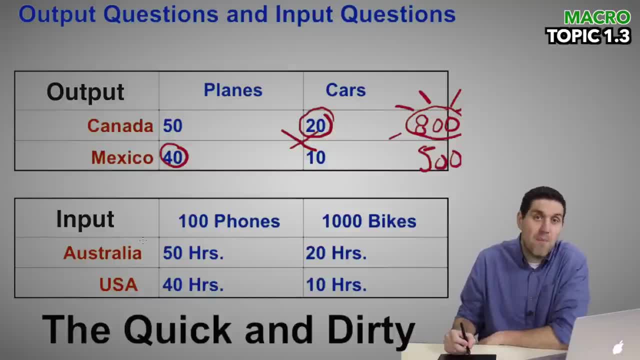 And it is quick and it is dirty. Now let's go down here. except remember we're doing an input question, So we're doing the same thing. It's 50, right here, times 10, which we already said is 500. 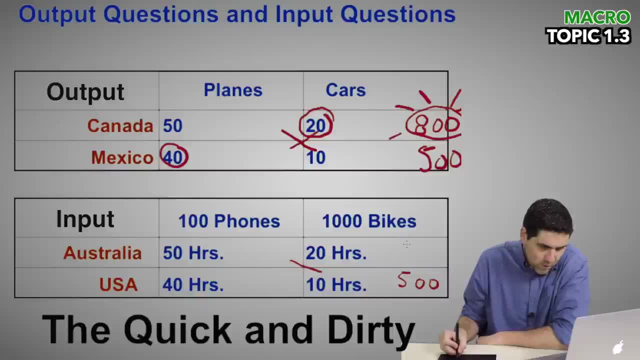 Or it's going to be the other option, which is 40 times 20,, which is 800.. So which one's the right option? Well, it's definitely 500.. Now you're going to use less hours. You're going to use less hours to produce the phones and bikes. 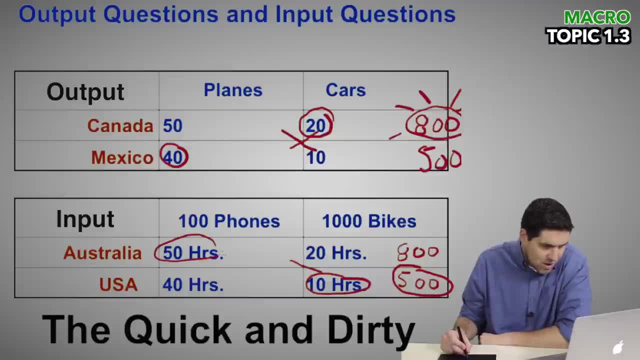 And so, no doubt about it, US should be producing the bikes, And, right here, Australia should be producing the phones Again. you could do all the other calculations if you wanted to, But this is a quick and dirty way to get the right answer. 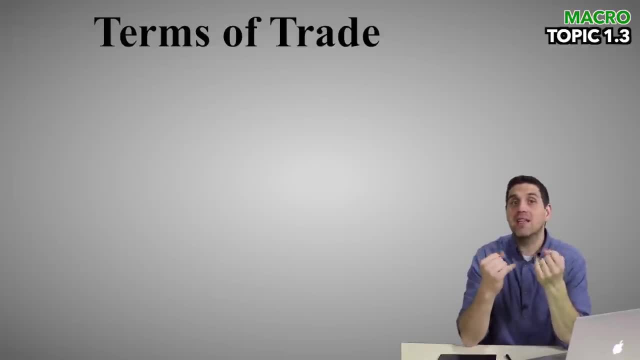 OK, how you doing You with me. You get the concepts All right, we're going to take it to the next level. We're going to learn this idea of what's called terms of trade. Terms of trade is that both countries can benefit, but they don't benefit at every single term. 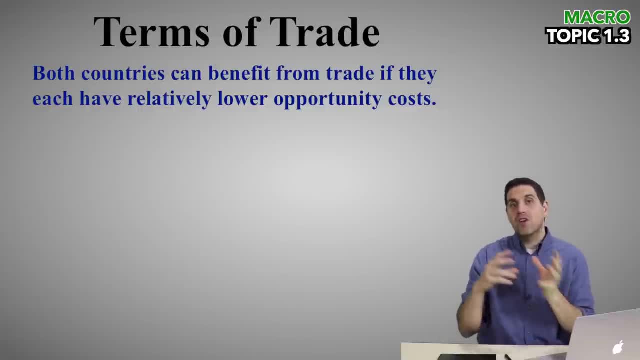 of trade. For example, they have to have a certain number of cars traded by a certain number of cars. They have to have a certain number of planes to benefit both countries. So an example I gave you earlier was one wheat for one and a half sugar for Brazil and the 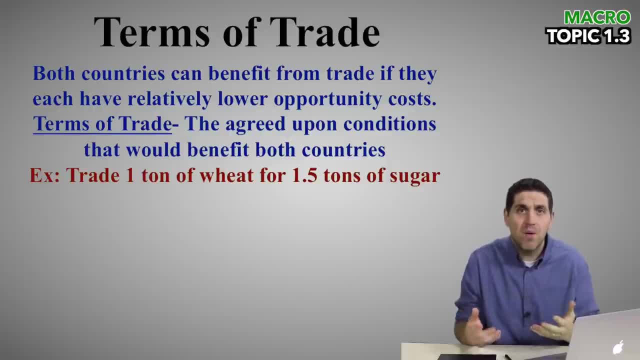 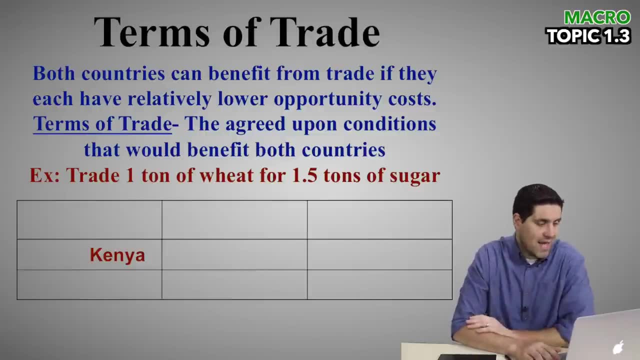 US would benefit both countries. How did I come up with that number? Well, that's what you're going to figure out Again. it's called terms of trade. It's agreed upon conditions that would benefit both countries. So we've got an example. question: 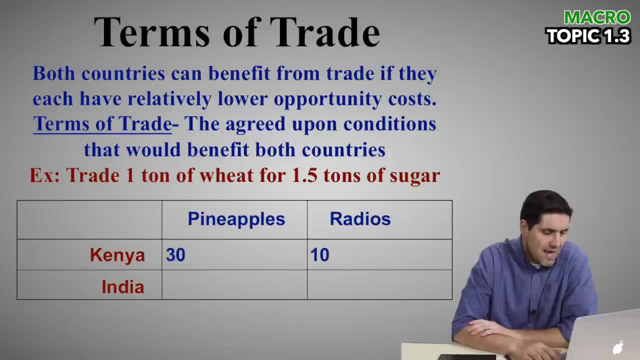 Kenya, India, pineapples radios 30,, 10,, 40, and 40.. What I want you to do right now is I want you to pause this video. I want you to figure out who has an absolute advantage in pineapples and radios. who has? 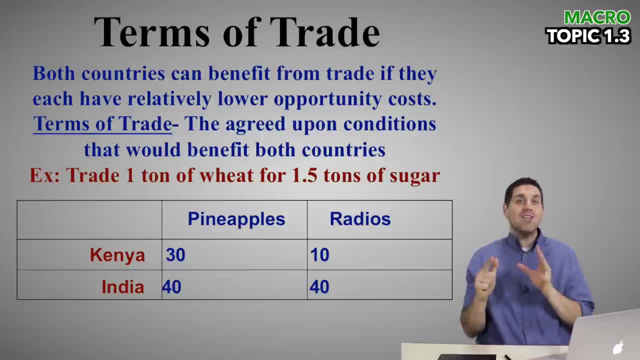 a comparative advantage in pineapples and radios. Also, I want you to try- I know you don't want to, I know you want to do the quick and dirty- but I want you to try to actually calculate the per unit opportunity cost for each one of those and figure out who has a lower opportunity. 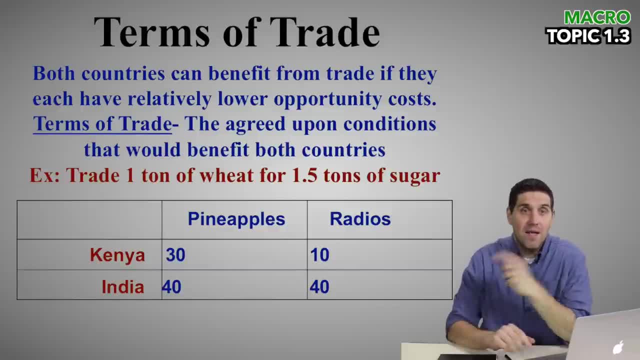 cost. All right, All right, Pause the video. See how you do. OK, you got it. Here we go For Kenya. each one of those pineapples cost one third of a radio they gave up, And each one of the radios cost three pineapples. 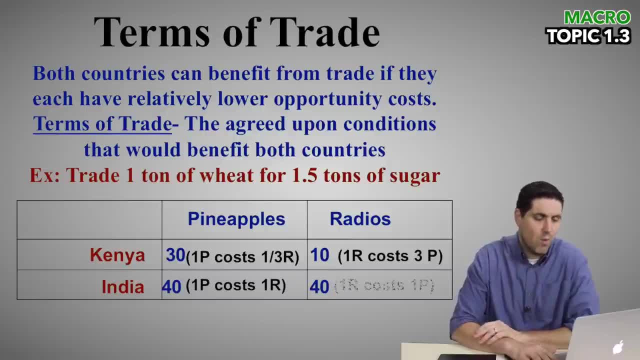 Now, India is pretty easy. It's: one pineapple costs one radio. One radio costs one pineapple. Now that we're there, It's time to figure out who has a comparative advantage, who has a lower opportunity cost. And it's easy because you have the numbers right. 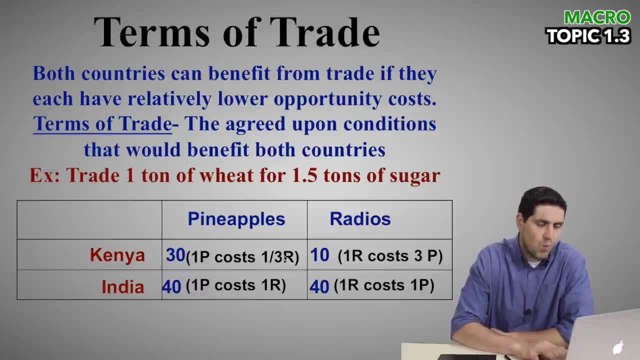 Pineapples one third. I'm sorry for Kenya. It costs one third of radio. For India it costs one radio. Who would you rather have producing the pineapples? The one that has a lower opportunity cost? So Kenya should produce pineapples. 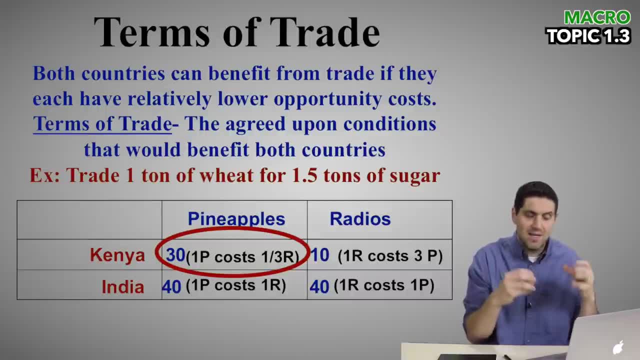 Again I'm circling, the one that has the lower opportunity cost, the one who should specialize in pineapples right? India has a lower opportunity cost, one compared to three lower opportunity costs in producing the radios, And so they have a comparative advantage. 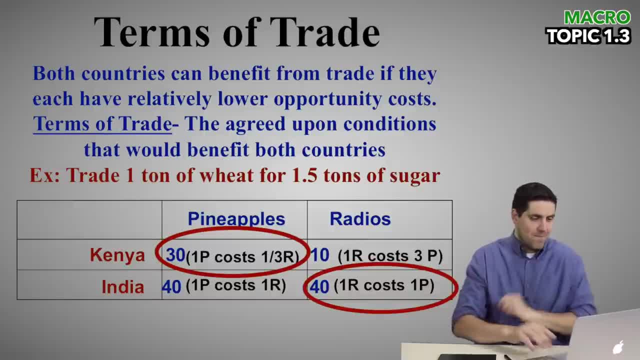 Now Let's use the quick and dirty to check to see if you're actually right. 30 times 40 gives you 1200.. 40 times 10 gives you 400.. 1200 is higher. That must be its right answer. 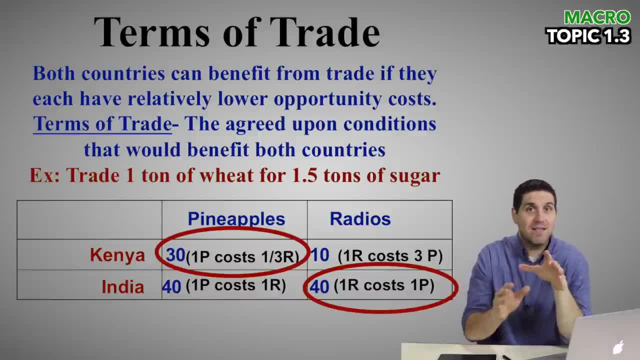 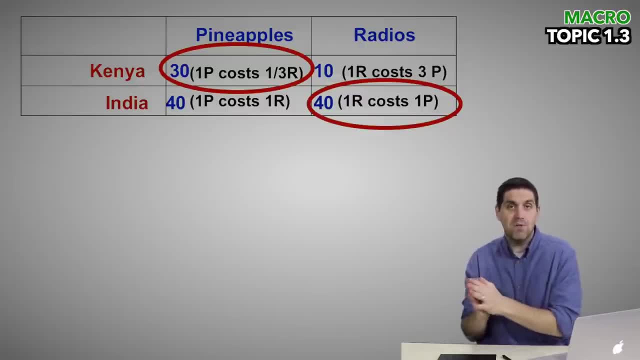 Done Output question. That's the quick and dirty, But we're not done. Remember we have to learn something called terms of trade. So we have to figure out each one radio can be traded for how many pineapples to benefit both countries. 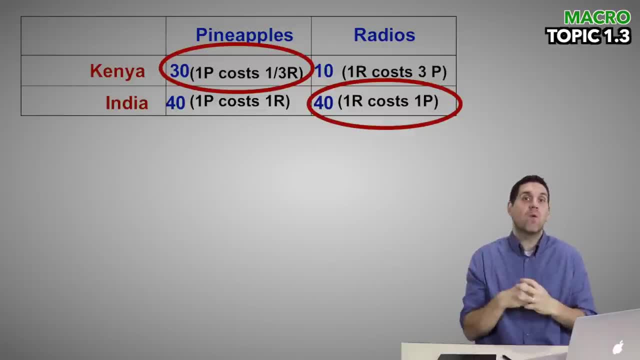 And I'll tell you right now: one radio for 10 pineapples is good for one country but not good for the other country. And one radio for like a half a pineapple is good for one country but not the other. So there's a range where you have to get the right number in that range. 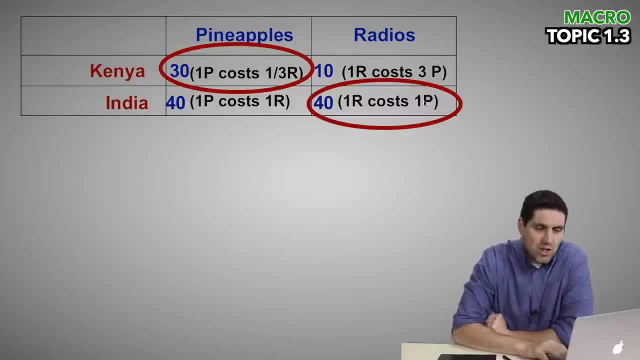 Now I'll help you out. Figure out how you get this. What you got to do is you look right here. This tells you what you calculated This pretty opportunity cost. The number for one radios for a certain number of pineapples has to be between three and. 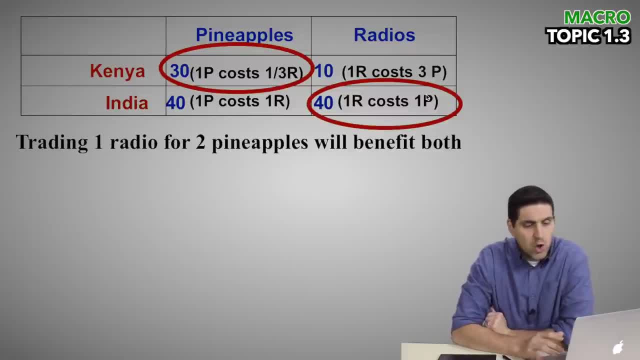 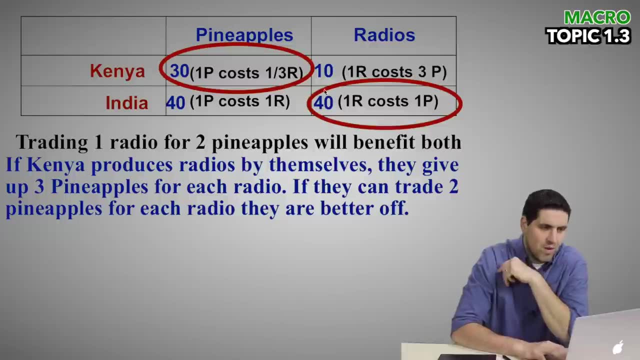 one right, For example, two would work. So one radio for two pineapples would benefit both countries. But why is that? Well, the reason why is this: If Can you, Kenya produces radios by themselves, So remember, Kenya is producing pineapples, right. 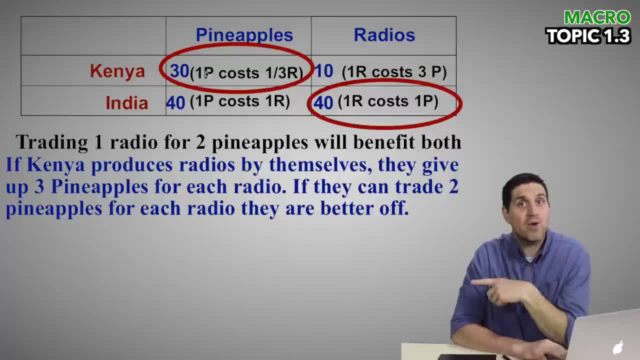 They're producing pineapples. If they want to produce radios, they're going to make them themselves, or they got to trade for them. If they make it themselves, how much does it cost them? Well, it costs them three pineapples, right. 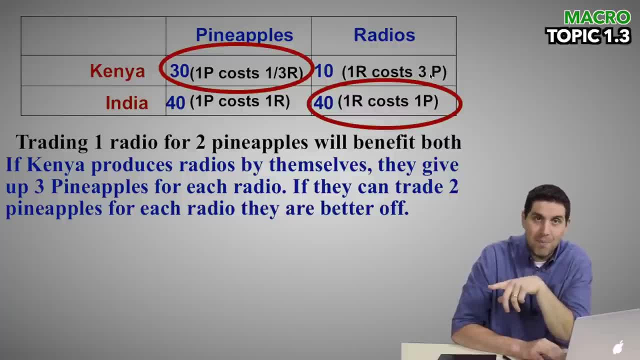 So if they produce themselves, cost them three. They'd rather trade two pineapples and get a radio than they would produce Give up three pineapples and get one radio by producing themselves. So this works for Kenya. They're like awesome. 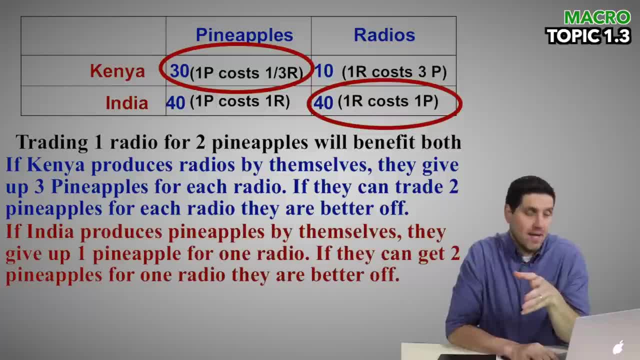 That's a great trade. It's better to give up two than three. But now let's look at India. right, They can produce pineapples on their own. If they do, it's going to cost them one radio, right. 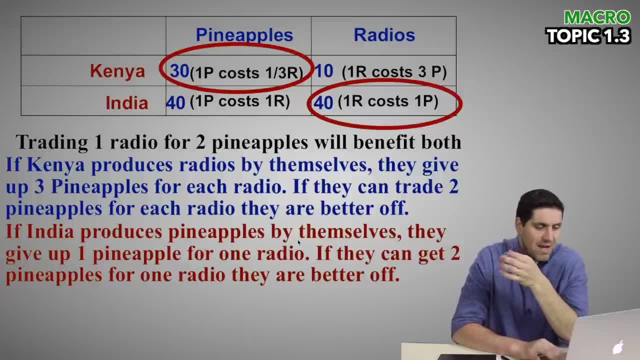 So they produce a pineapple and it's going to cost them one radio. But in this case they can give up one radio and get two pineapples. right, They give up one radio because they're specializing in radios. They can get two pineapples, as opposed to giving up a radio and getting only one pineapple. 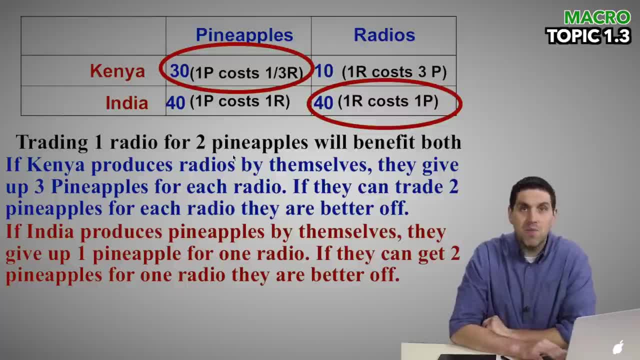 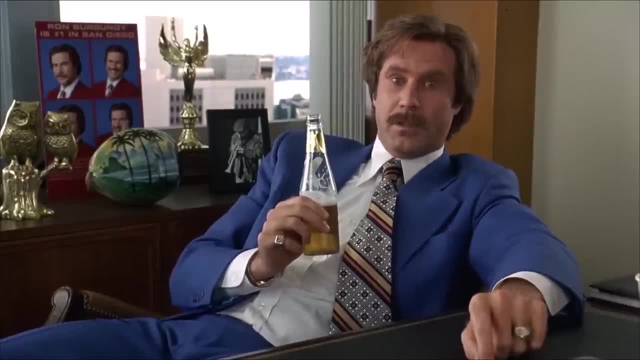 themselves. So in this case, one radio for two pineapples benefits both countries And that's a terms of trade that is great for both of them. Boy, that escalated quickly. Okay, That was a whole lot, And for many students, compare advantage is the hardest thing for them to learn, especially. 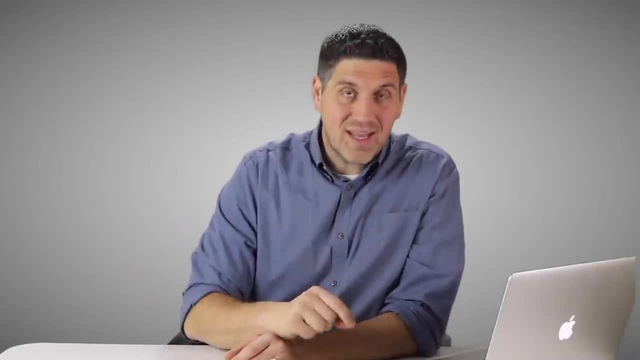 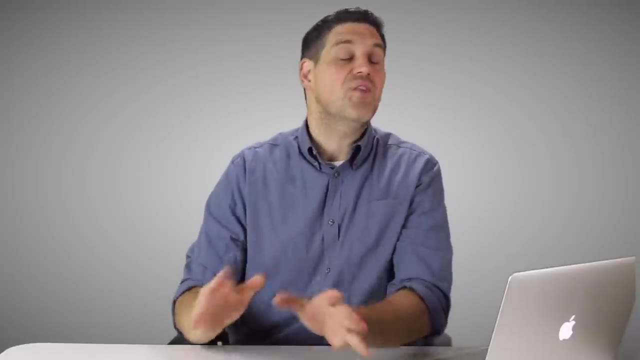 here in unit one. So right now it's time to stop and fill out the unit study guide on the ultimate review packet to verify you're actually getting it. So try to output question. try to input question. calculate the terms of trade. See if you can actually do this right now. 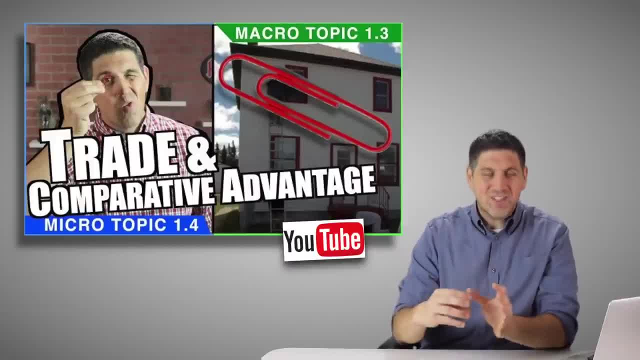 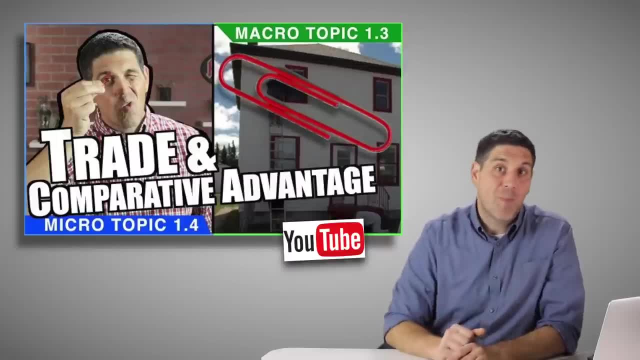 And if you get all the answers right, Awesome. Keep watching this video, but if you don't understand it, go back to YouTube. Watch my topic video that covers a concept over again and make sure you understand. compare badge. then start the video back up. 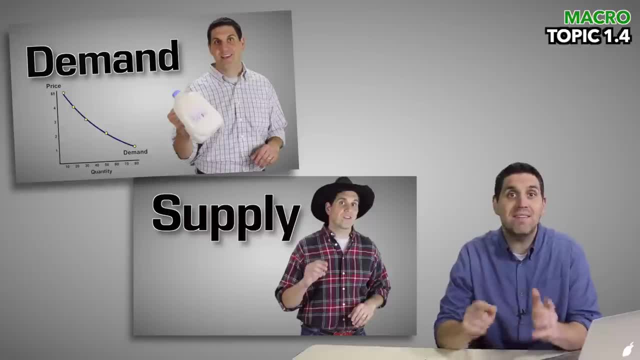 All right, let's do this Now. the last thing we're going to do in this unit is talk about demand and supply in a market. Now, this is super important. I've made awesome videos on this already, covering the topic, So right now I'm going to do a pretty fast summary. 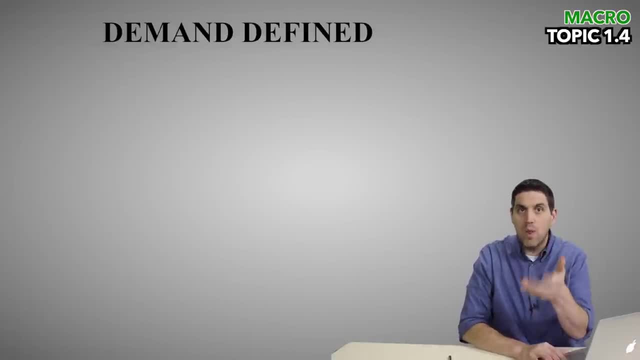 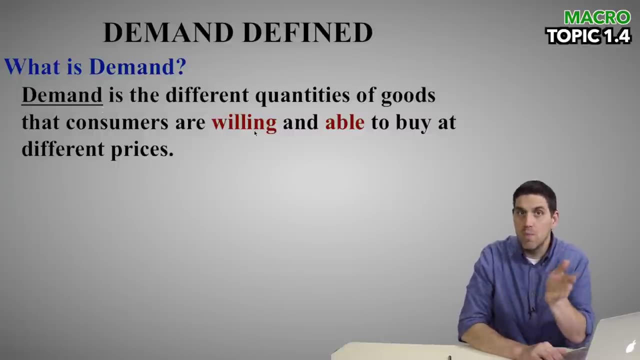 I'm going quick right now. Demand: You already know this is what consumers are willing and able to pay, And there's a relationship between price and quantity. So the definition of demand, demand is a different quantities of goods that consumers are willing and able to pay at different prices. 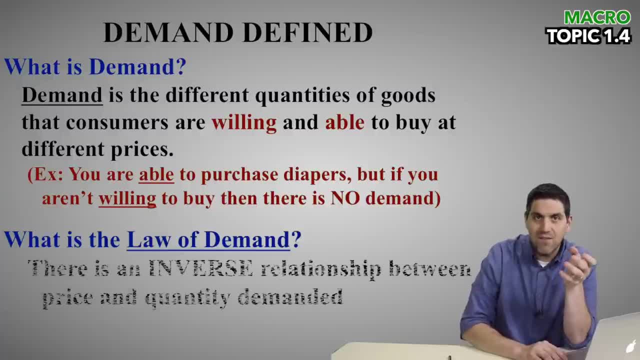 Now there's something called The law of demand. The law of demand shows you that there's an inverse relationship between price and quantity demanded. when the price goes up for stuff, People buy less of that stuff, and the price goes down, People buy more. 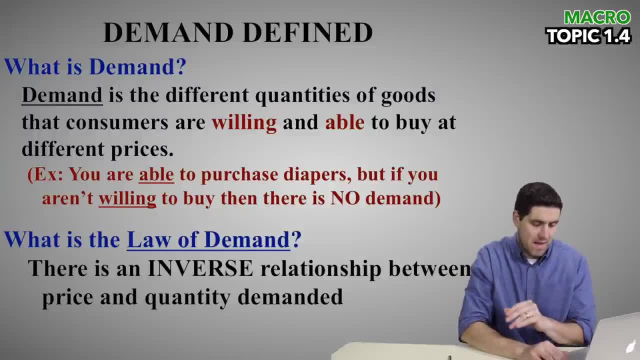 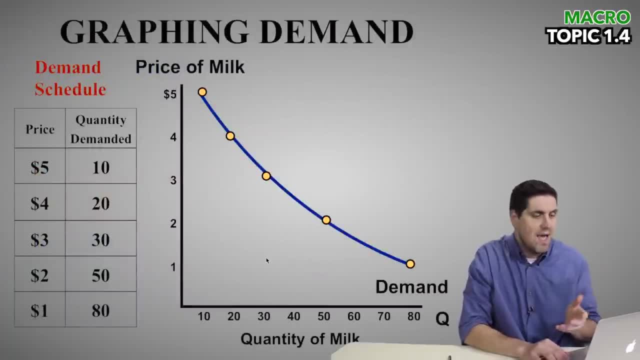 It's pretty standard, Everyone knows it. That's the concept. Again, it's called the law of demand. Now that means that there's a demand curve on a graph. If you have price and quantity, there's a demand curve. In this case, let's use milk. 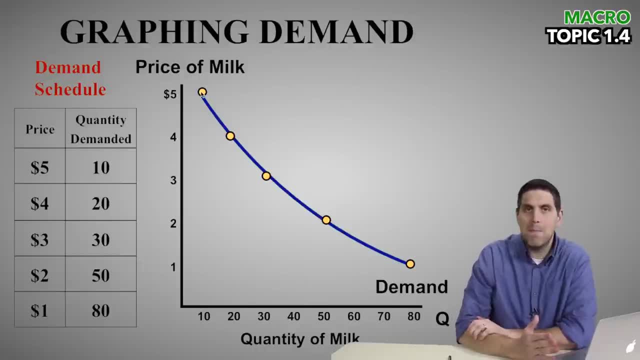 If the price is up here, right right there at five, not very many people are going to want to buy milk. but if the price is lower, at only $1 per gallon, the people are going to buy more, And so that downward sloping curve. 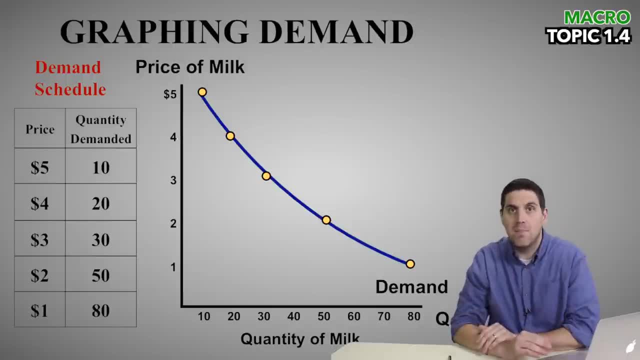 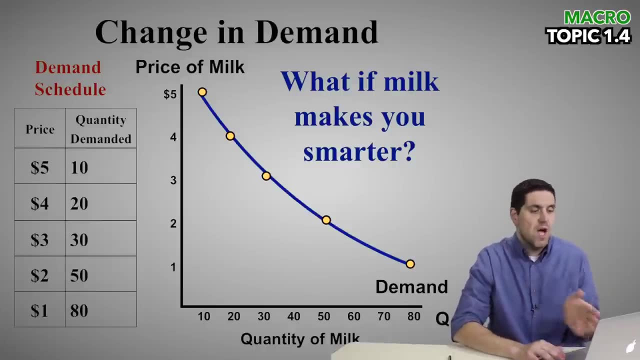 It shows you an inverse relationship between price and the quantity demanded. but a demand curve can also shift. So if there's some other change other than price, the demand curve can shift right or left. So if milk makes you smarter, there's some study that comes out says milk makes you. 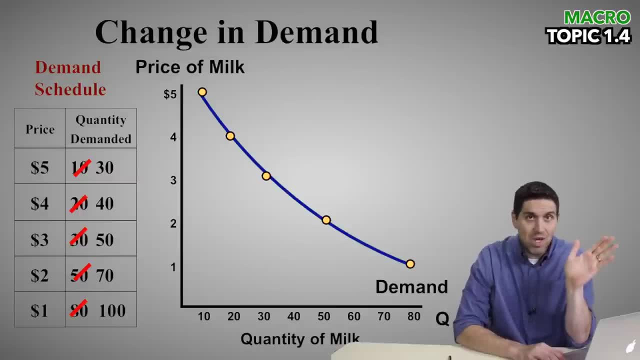 smarter. People want more milk, right, And so at every single price people are going to want more milk. The entire curve will shift to the right. That's called an increase in demand. Now, if something else happens- let's say milk causes baldness- then that means less. 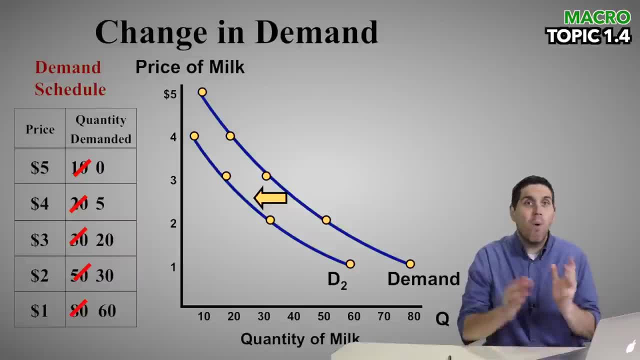 people want to buy milk, The entire curve would shift To the left. Now, it's important to understand this idea of curves shifting right and shifting left. You're going to do it a whole lot in this class, Now how about this one? 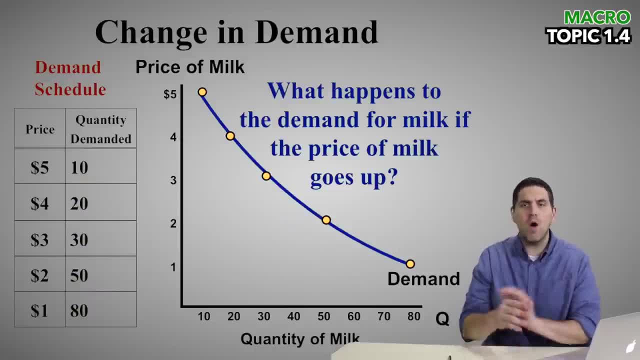 What happens to the demand for milk if the price goes up? Well, you might be like, oh, the price goes up, Demand will go down. No, no, no, The quantity demanded goes down. Remember, if the price goes up, the quantity demanded goes down. 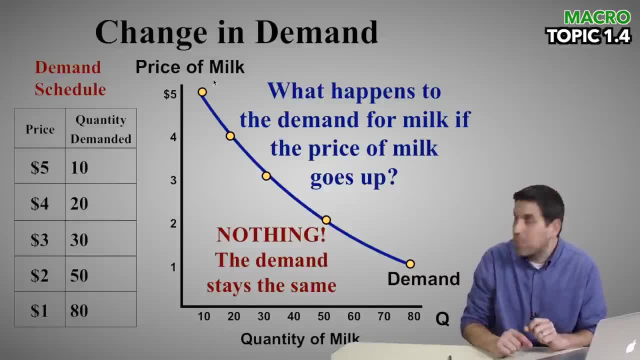 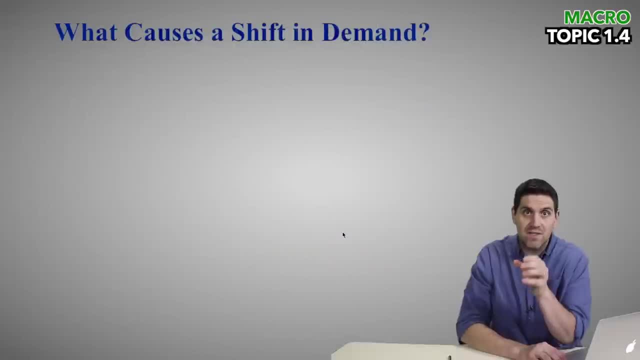 So the curve wouldn't shift. It would just be a movement along the curve. So the price would go up, right, The quantity would decrease. Movement along the curve, not a shift in the curve. Now, what shifts the curve is things other than price. 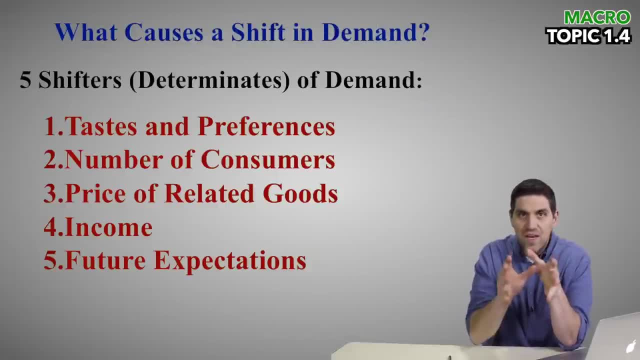 In fact, here's the list: Five shifters of demand. The video that I was talking about covers these really well, goes in more details and it gives you more practice than I'm going to do right here. But those are the shifters of demand. 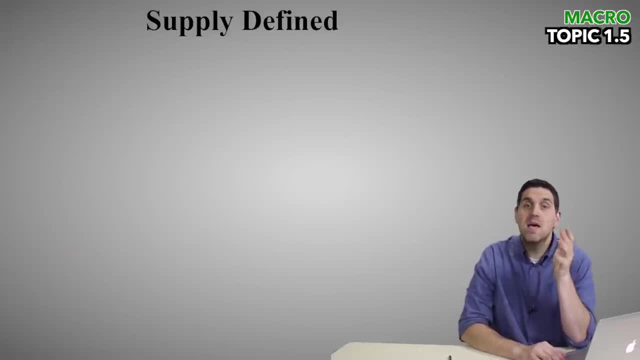 That's what causes the curve to shift. Now let's look at the other side: supply. Supply is the different quantities of goods that producers are willing and able to sell at different prices, And, of course, there's also the law of supply. 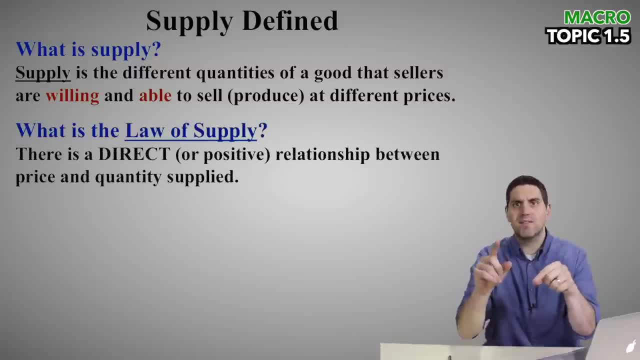 The law of supply says: when the price goes up, producers want to produce more- right, Because they can make more profit. So price goes up, I'm going to produce more. Price goes down, I'm going to produce less. That means we have a curve. 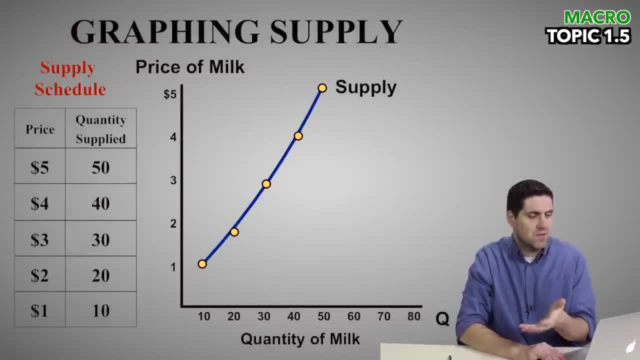 What's the curve look like? Well, it's an upward curve. It's an upward sloping curve. right Supply curve is upward sloping. When the price is low for milk, producers don't want to produce very many. The price goes up for milk, they want to produce a whole lot more. 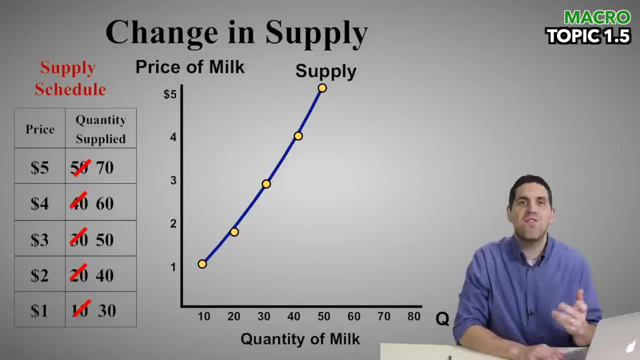 But it can also shift right. So, for example, if there's a new technology that produces milk faster, that means the entire supply curve would shift to the right. If a bunch of cows die, that would decrease supply and shift it to the left. 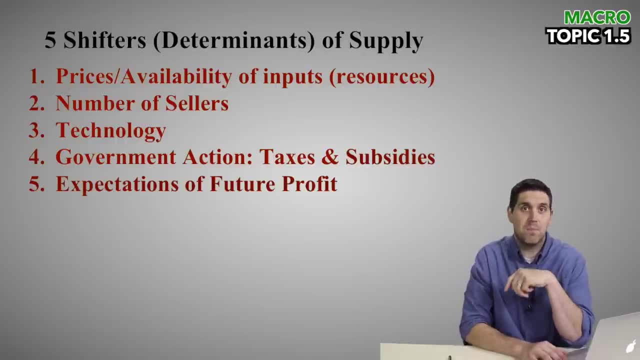 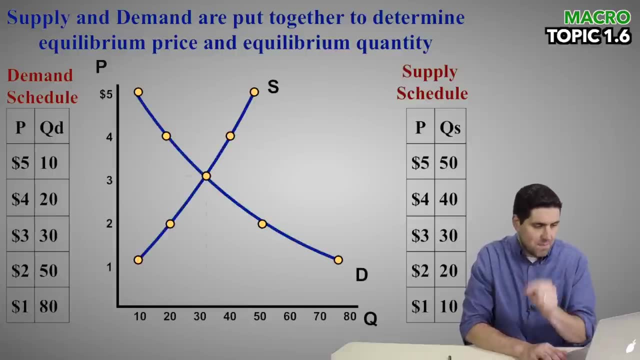 Remember: increase is always right. Decrease is always left when it comes to supply and demand. Now that we understand that, let's put supply and demand together. Right here we get the idea of equilibrium. Demand hits supply at, in this case, $3 for a gallon of milk. 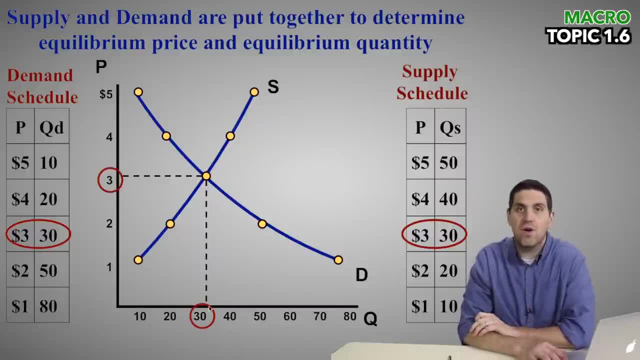 And then the quantity is dot dot down right there, in this case at $30.. Now that's the price and quantity that's going to happen in the market at any given time. But there could be something weird happening, For example if the price was really high, let's say up here at $4, then we're at disequilibrium. 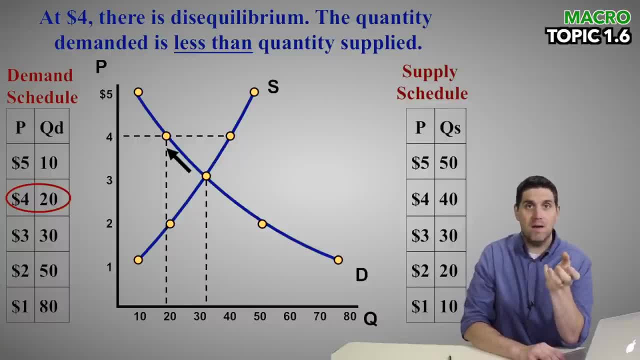 In this case the quantity supplied is greater than the quantity demanded, right? So if the price goes up, people don't want to buy it, So the quantity demanded goes down. But producers want to produce more, And so the quantity supply goes up. 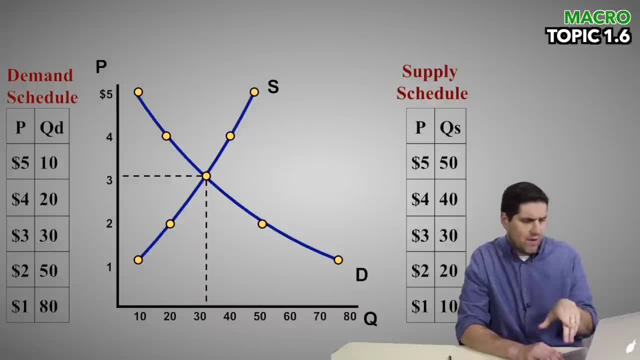 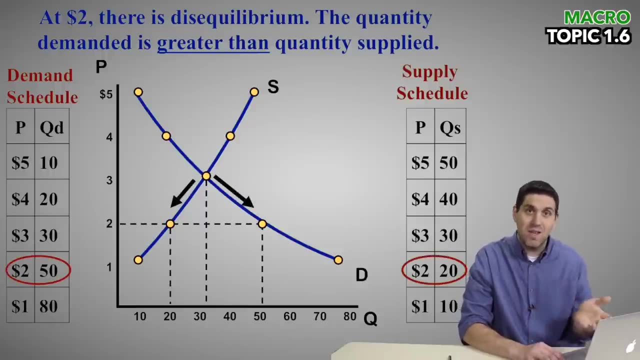 The result is something called a surplus. Now, if the price was really low- let's say down here at $2, then people want to buy more of it, So the quantity demand goes up. But if the price is low, producers don't want to produce very many, so they'll produce less. 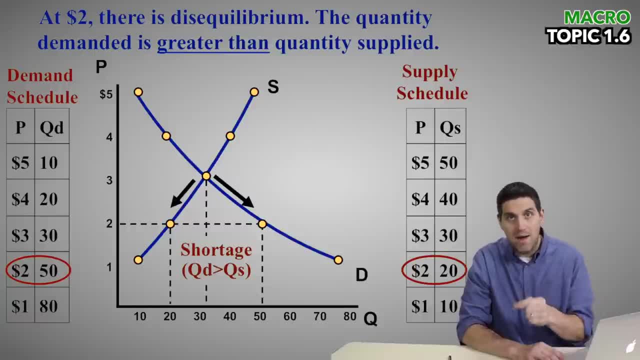 Quantity supplied will go down. The result is a shortage, right, The quantity demanded is greater than the quantity supplied. That's the idea of a shortage. Now, a surplus and a shortage might happen in the market, but they don't stay that way. 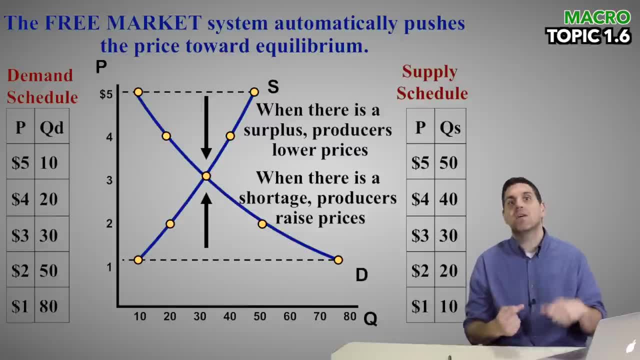 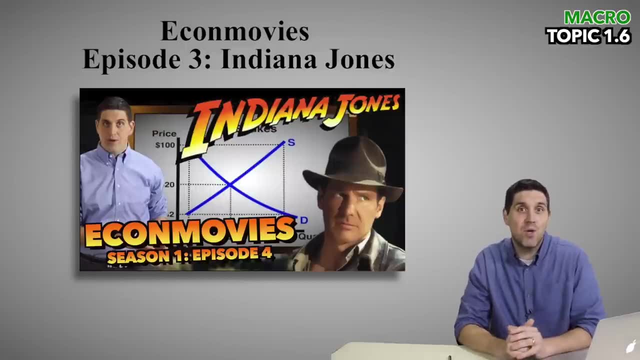 Equilibrium happens for a reason: A shortage pushes the prices up, A surplus pushes the prices down, And a market should be at equilibrium, unless something weird is happening Now. if you haven't seen it yet, you should. It's the Indiana Jones econ movies. 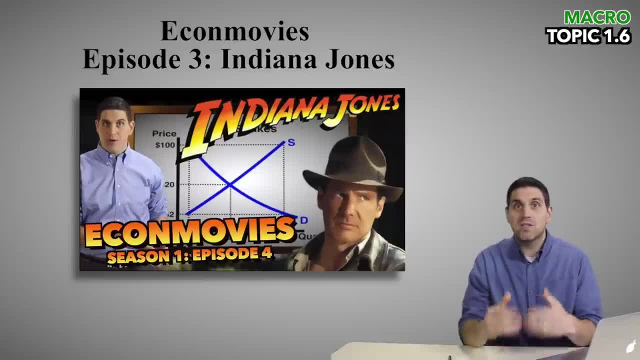 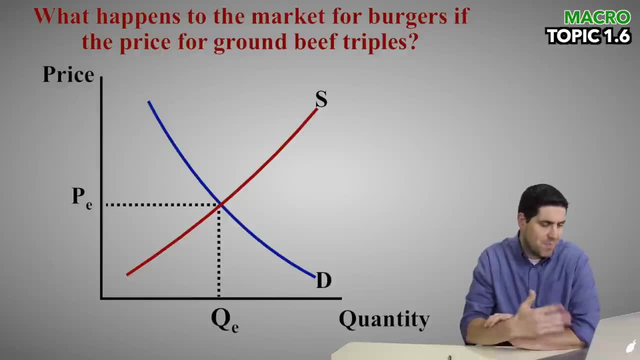 It talks about supply and demand and shifters. It's pretty good stuff And it introduces some of the ideas that you need to be able to do, like the idea of shifting a curve. So here we have an equilibrium for burgers: Demand, supply and some price, PE and quantity QE. 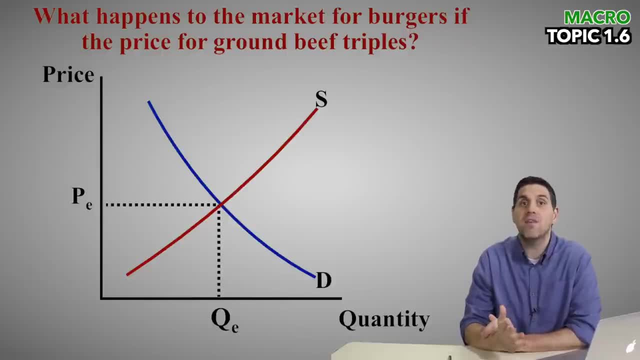 And the question is: what happens to the market for burgers if the price of ground beef triples? So if the price of a key resource triples, it doesn't affect demand, It affects supply, And if it triples that means supply is going to decrease. 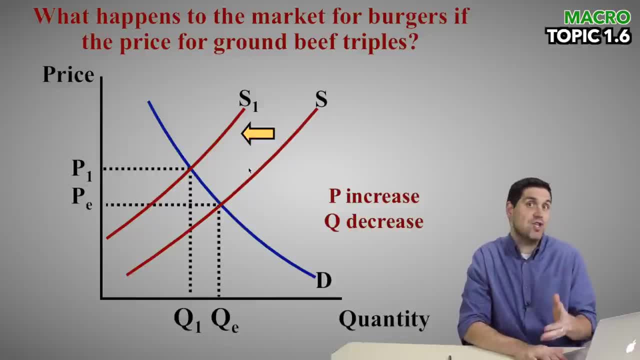 They can't produce as much as they could before. When supply decreases, it shifts To the left, and you just read the graph: right, Right there. it tells you the price went up and the quantity went down. right, Price went up, quantity went down. 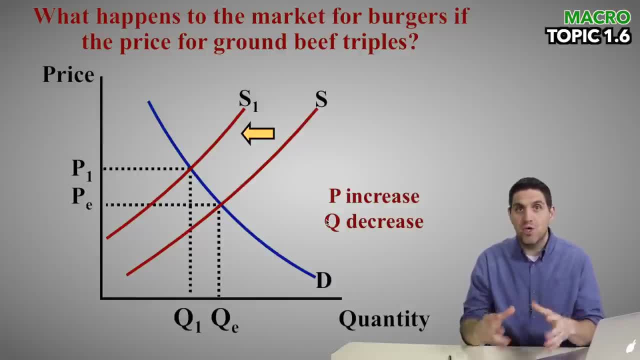 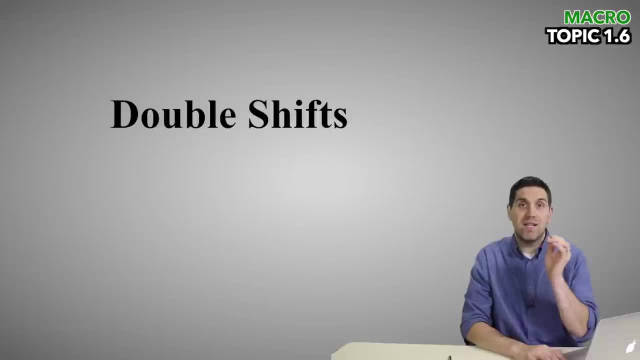 And that tells you what happened to the market. Understand this general concept. You can do a whole lot more of this stuff when it comes to aggregate demand and aggregate supply later in macroeconomics. Another key concept you have to understand is the idea of double shifts, right. 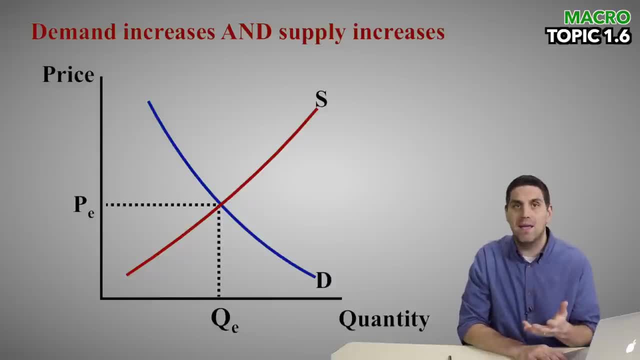 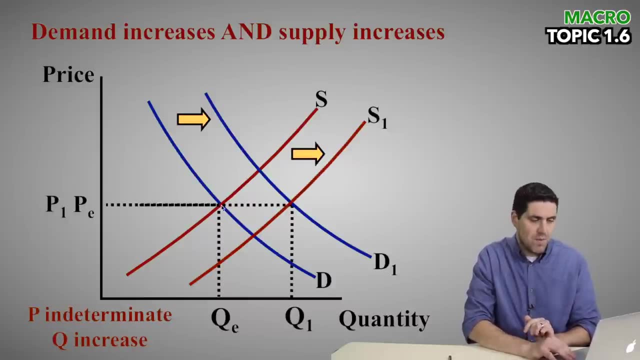 So suppose the demand increased, at the same time supply increased. Well, demand curve shift to the right, Supply curve shift to the right. We started equilibrium right here. We ended the equilibrium right here, right. So that tells you what happened on the graph. 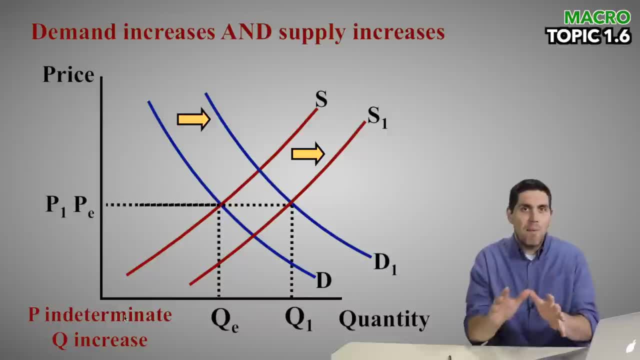 And now it looks like quantity went up and price stayed the same. But remember, when it comes to double shifts, the idea of price is indeterminate. You can't tell. It depends on the severity of the shift. Now I've got another video explaining that concept called double shifts. 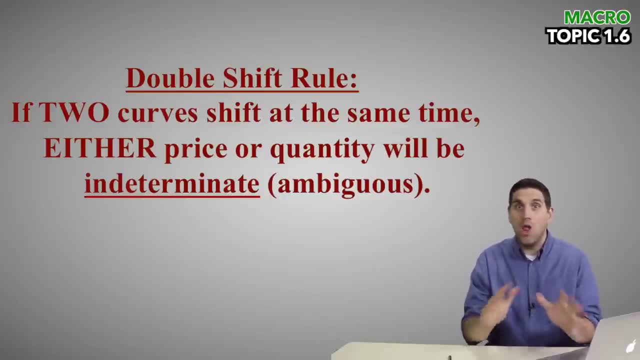 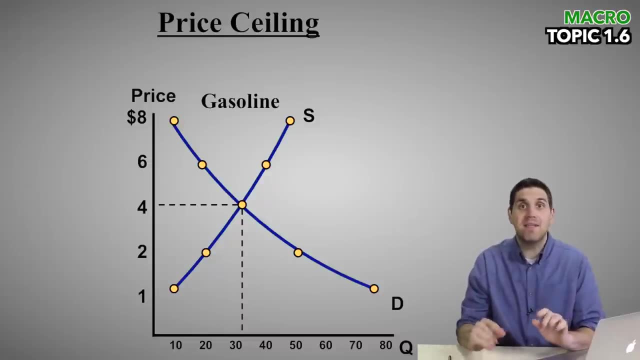 But just right now, remember there's a key rule, And the key rule is always: when two curves shift at the same time, either price or quantity is going to be indeterminate. The last thing I want to talk about is the idea of ceilings and floors. 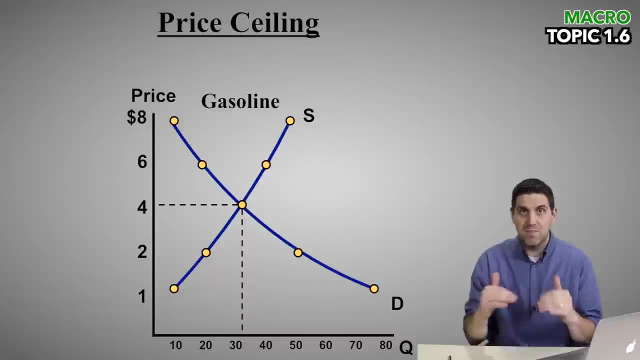 The government can mess up a market. They can come in and set a price at a different spot or do some sort of regulation. In this case, a price ceiling is a maximum legal price a seller can charge for a product right, And so a price ceiling is below equilibrium when it's binding.